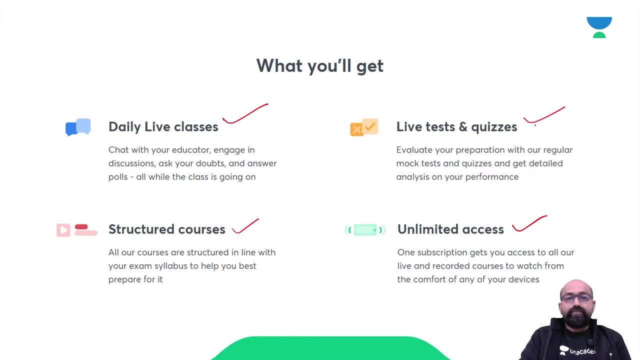 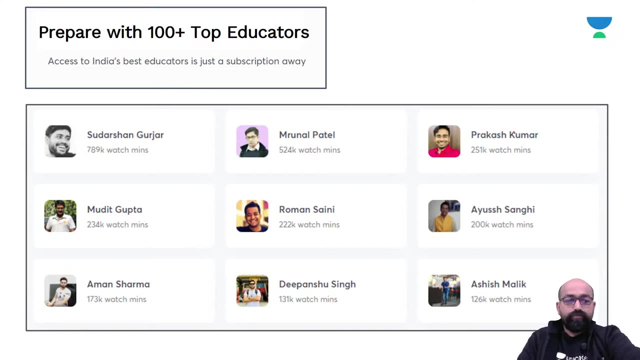 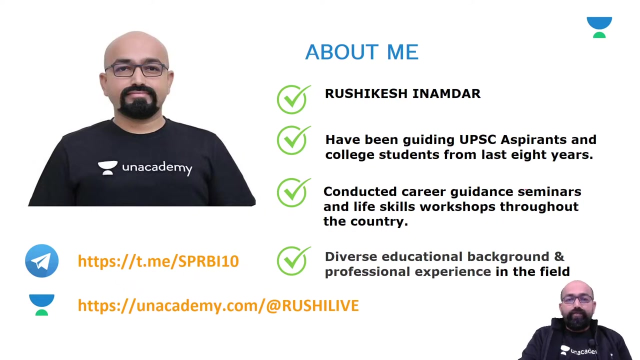 with unlimited mock tests. Yes, in today's lecture we'll see indoor air pollution. Yes, friends, we 100 plus top educators will guide you throughout the preparation of civil services examination. I'm having experience more than eight years in the field of guiding UPSC aspirants You. 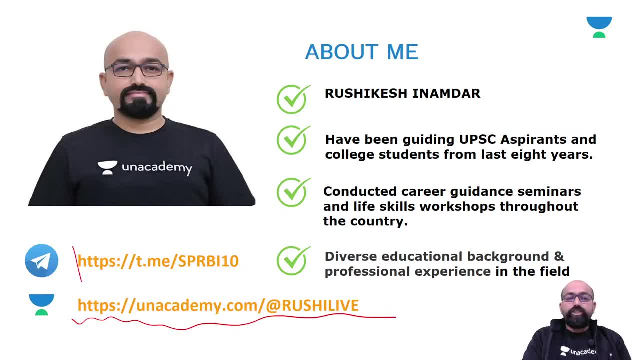 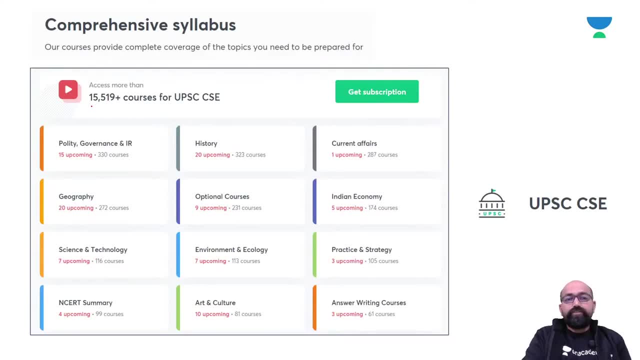 can follow me on Unacademy and you can join our Telegram group using this link. Yes, those aspirants are looking for any particular module-wise courses. We have 15,000 plus courses available on our platform. Yes, friends, we 100 plus top educators will guide you throughout the preparation of civil. 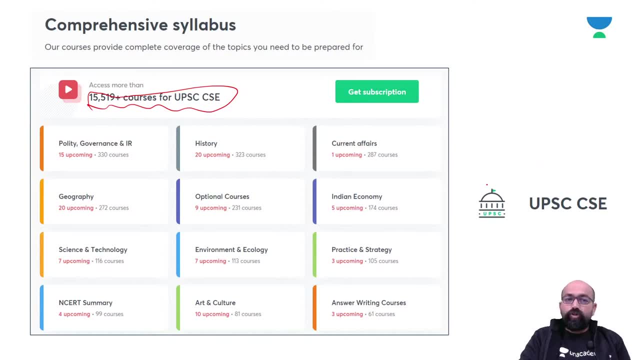 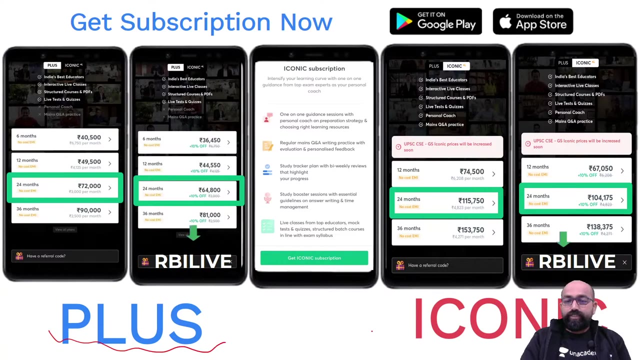 service examination If the Along with international relations, Indian economy, geography, environment and ecology, analgesic and many more. so please start your preparation with Unacademy. Yes, we have options for plus and iconic subscription, where you will get proper structured courses. 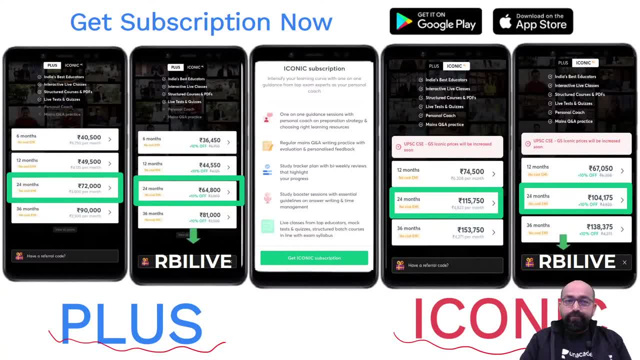 And those aspirants are preparing for their graduation or degree, So please proceed with your full-time follow-up as we close this webinar channel and open degree, they can opt for iconic subscription means. in this subscription, you will get personal coach along with study planner and do not. 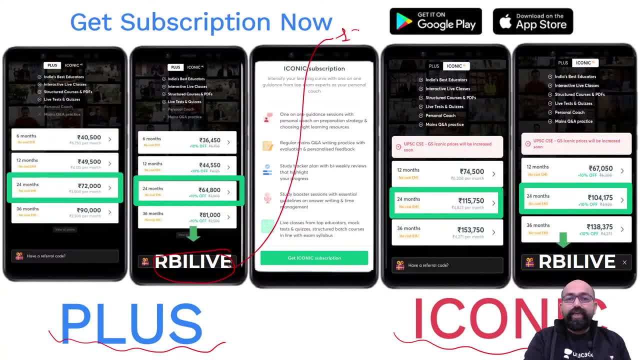 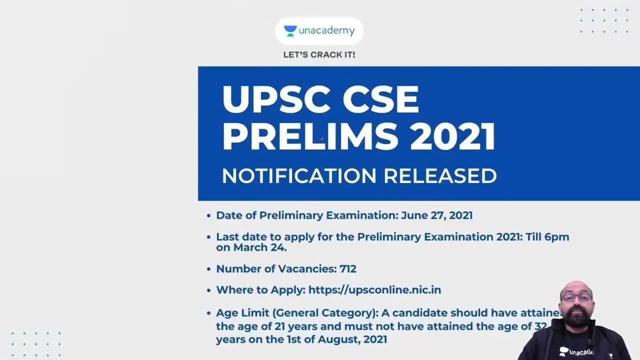 forget to use code RBI life to get 10% discount on your subscription. yes, you can apply this referral code RBI life on plus or iconic subscription as well. yes, yes, friends, as everyone aware about notification of CSE 2021 prelips is already published. yes, so 27th June is the exam date and last date for the 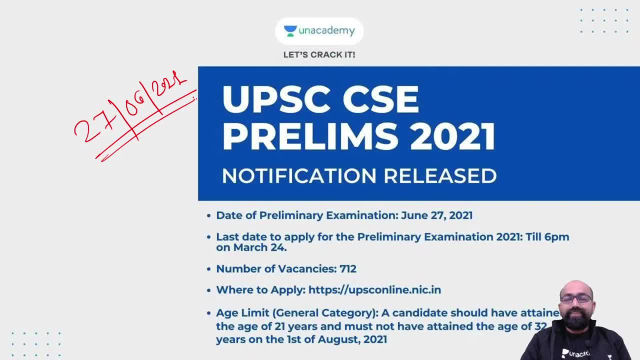 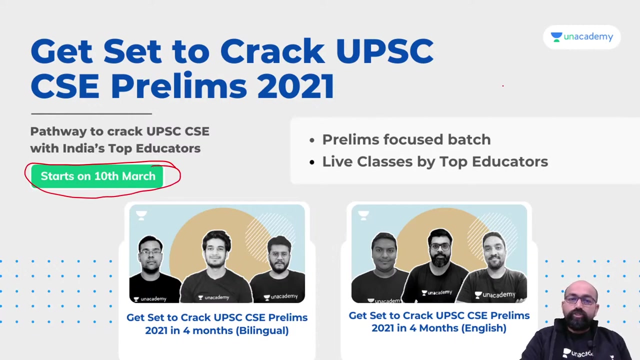 apply for the preliminary examination in is 24th March. yes, guys, you can visit the website of UPSC for apply preliminary 2021: prelims exam 2021. yes, and all these details regarding vacancies and eligibility criteria. yes, guys, we are going to start new batches from 10th March, so hurry up and enroll. 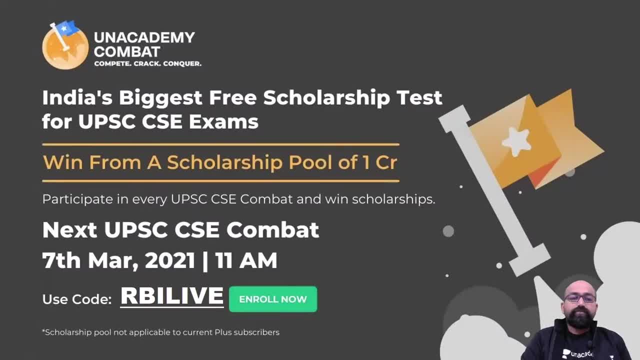 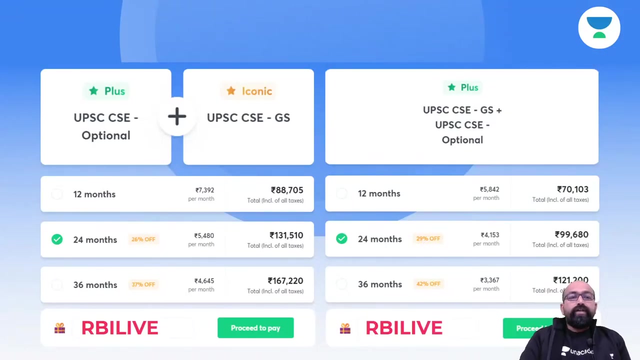 yourself for these batches. yes, friends. we have next an academic combat scheduled on 7th March in the morning, 11 am. so do not forget to register yourself using code RBI like yes. so hurry up and register yourself for the unacademy combat. yes, friends. these are the subscription options. 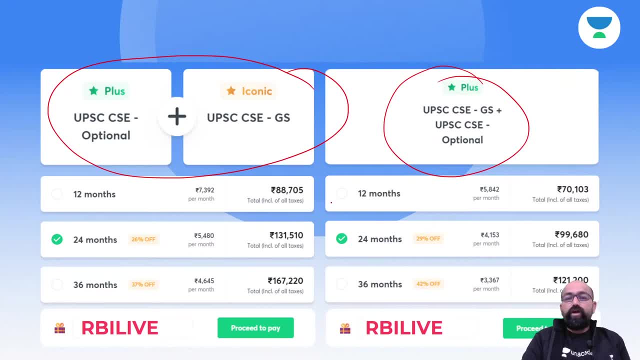 available for you again. you have option to opt for oneità match for now. HEFSimbcaura Friedland Stokartasulcom. please register a subject surely under holicovid test, and add info to this video. year, two year or three year subscription and you can use code RBI life to get 10%. 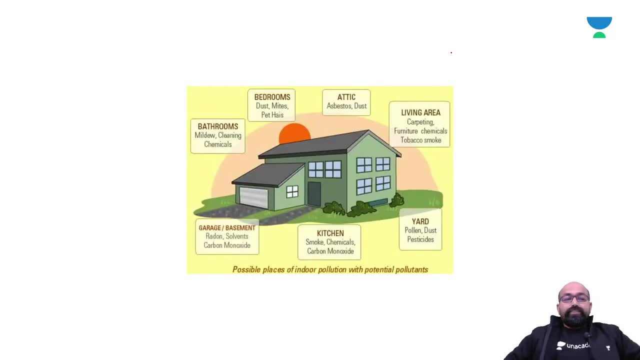 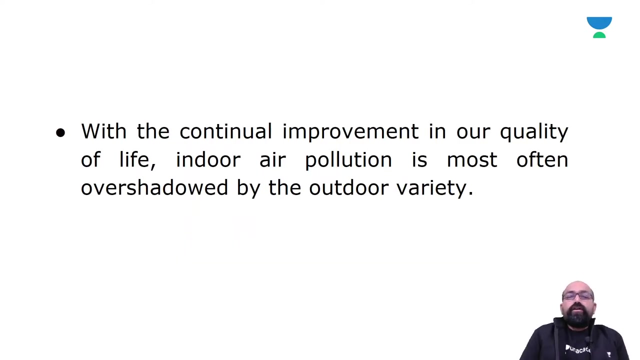 discount. yes, now in today's session we'll see indoor air pollution. now tell me anyone, anyone of you, what is mean by indoor air pollution. yes, see, this picture is talked about in deep sense, in depth, about indoor air pollution. yes, friends, now so with the why it is in news, because with the continuous pollution of consumer goods. all mean, as you saw earlier earlier today, reduced DY, buy, buy, buy and buy. with system久many is diminishing of fat down square effective given and maximum increase of Houttuynia. cordial appreciation C, which again thank me so much. the video and thank you, my fortune and spices, this will be. 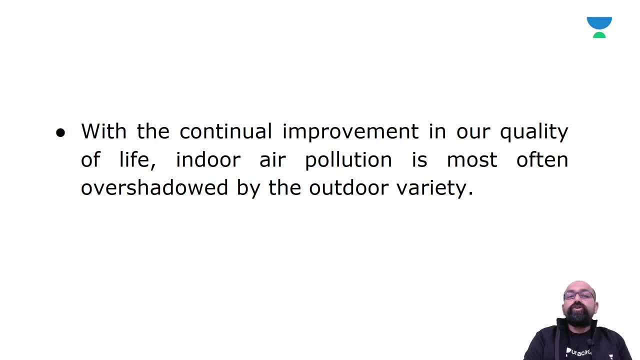 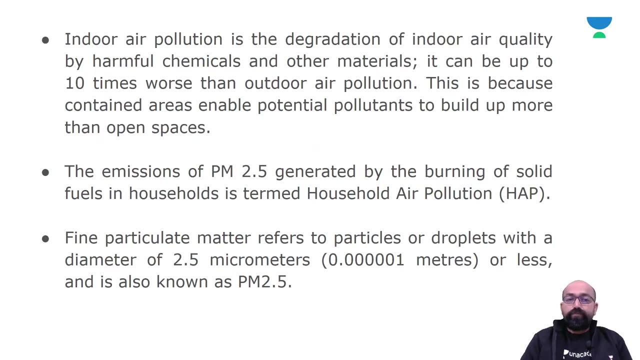 improvement in our quality of life. indoor air pollution is most often overshadowed by the outdoor variety. yes, means so. in the indoor air pollution is the degradation of indoor air quality. yes, the degradation of indoor air quality by harmful chemicals and other materials. so it can be up to ten times. 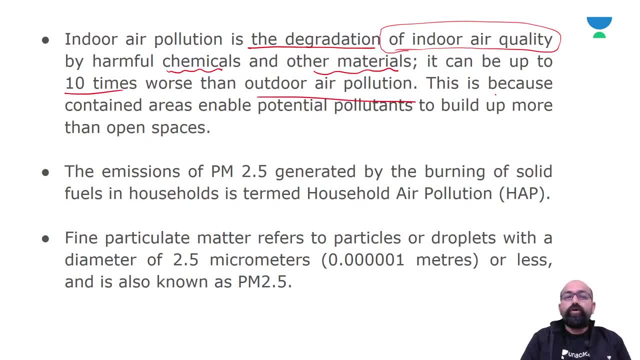 worse than outdoor air pollution. so this is because content areas enable potential pollutants to be polluted by harmful chemicals. so this is because to build up more than open spaces, yes, so what is mean by indoor air pollution? so, though, which is the degradation of indoor air quality, and this degradation 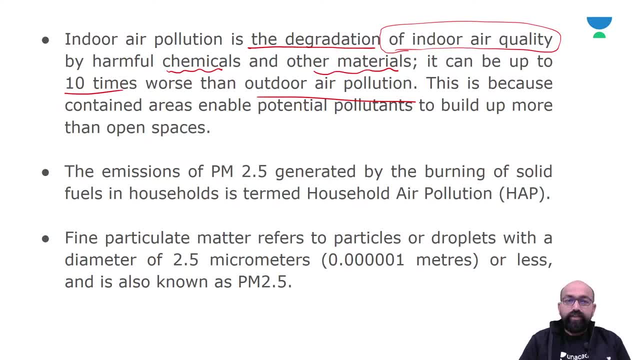 by harmful chemicals and other materials. now, the emission of PM 2.5 generated by the burning of solid fuels in households is termed HAP- household air pollution. yes, guys, I hope everyone is aware about HAP household air pollution. yes, now fine. particulate matter refers to particles, or 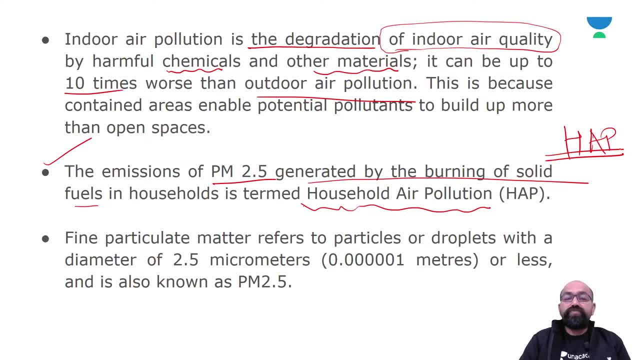 droplets with a diameter of 2.5 micrometers or less is also known as PM 2.5. Yes, as we know during last few years, we are facing a severe air pollution in northern part of our country, like Delhi and nearby places facing air pollution. 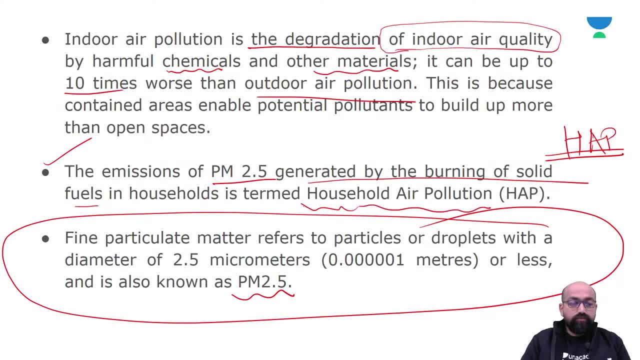 Yes, before that. Yes, Vijay, everyone is waiting for that result, So keep patience. Definitely, As soon as possible, UPSC will declare his result of mains, So keep updating their website, please, And definitely will announce through our platform as well. 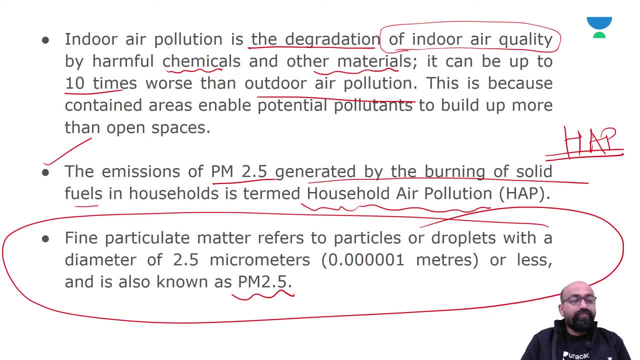 Such important events? Yes, So come to the point. Today we are studying indoor air pollution. So what is mean by PM 2.5 particles? So the fine particles refers to our particles, or droplets with a diameter of 2.5 micrometers or less is known as PM 2.5. 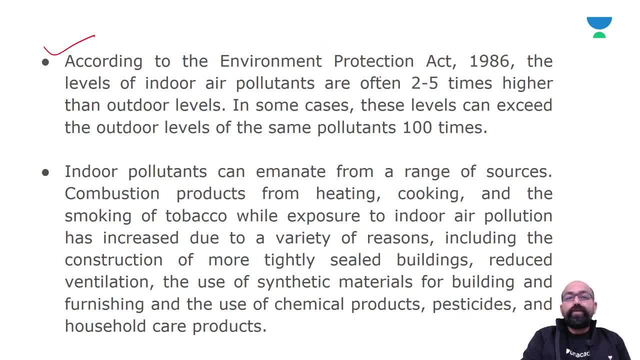 Now, according to the Environment Protection Act 1986, the levels of indoor air pollutant are often two to five times higher than outdoor levels. So in some cases these levels can exceed the outdoor levels of the same pollutant hundred times. Yes, this is the observation by Environment Protection Act 1986. 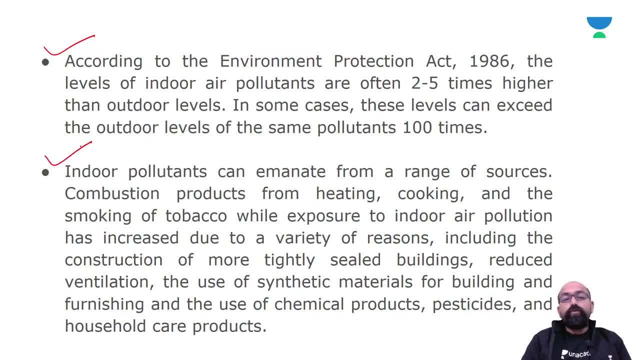 Next, indoor pollutants can demand from a range of sources, So combustion of products from heating, cooking and the smoking of tobacco. While exposure to indoor air pollution has increased due to a variety of reasons, including the construction of more tightly sealed buildings, reduced ventilation. 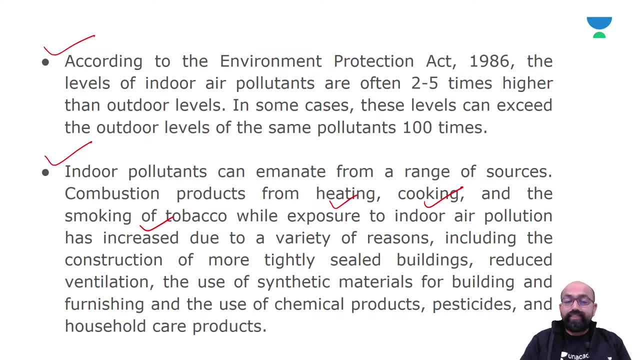 Yes. The use of synthetic materials for building and furnishing and the use of chemical products, pesticides and household care products: Yes. So see the reasons for the indoor pollutants Then. according to WHO, around 3 billion people, Mostly women. 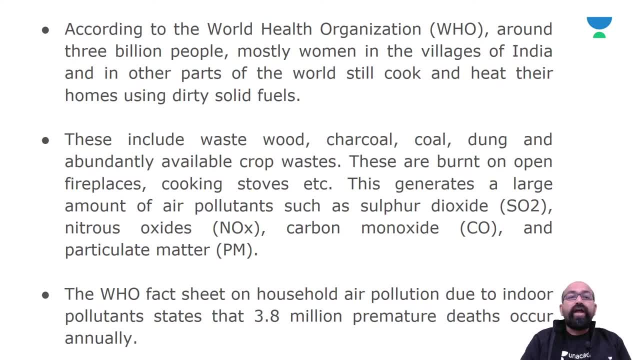 Yes, Mostly women in the villages of India and other parts of the world still cook and heat their homes using dirty solid fuels. Yes, This is the report or observation by WHO where they observed that 3 billion people, mostly women, women in the villages of India and in other parts of the world still cook and heat their 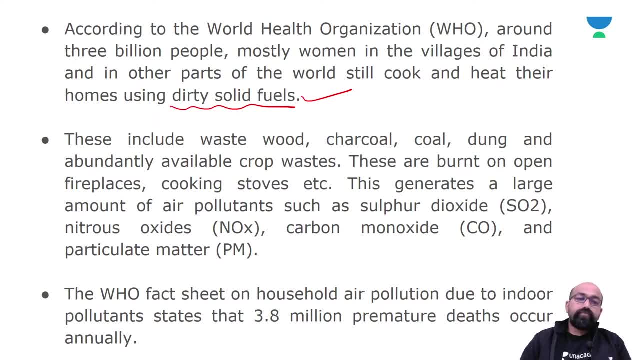 homes using dirty solid fuels. Now this includes wood, charcoal, coal dung and abundantly available crop wastes. yes, So these are burned on open fireplaces, cooking stoves, etc. So this activity generates a large amount of air pollution, such as SO2, sulfur dioxide. 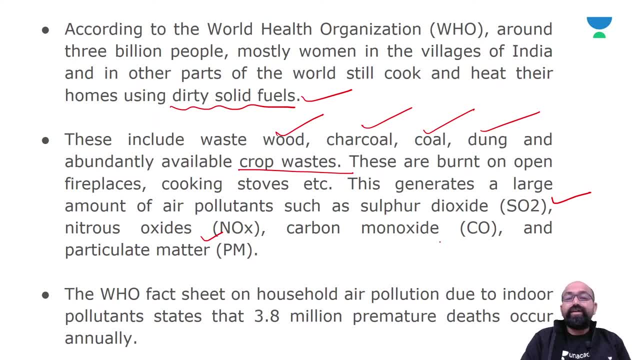 NOx, nitrous oxide, carbon monoxide and particulate matter, that is, PM. Now, the WHO fact sheet on household air pollution Due to indoor pollutants states that 3.8 million premature deaths occur annually. yes, So the 3.8 million premature death occurs annually due to indoor pollutants? yes, 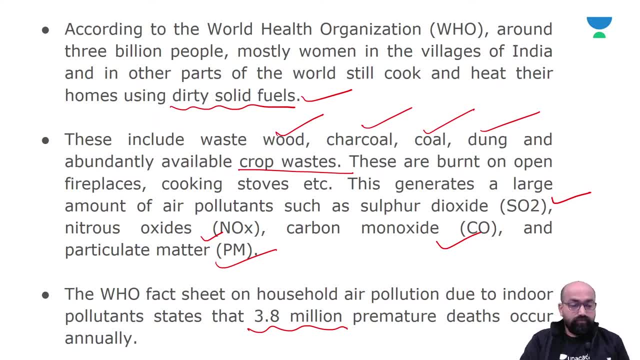 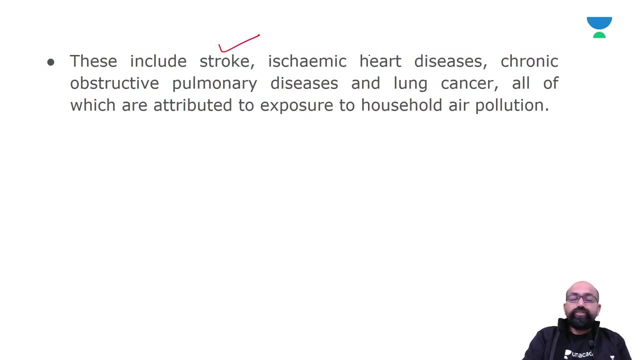 Okay, So these include. reason for this date includes stroke, ischemic heart diseases, chronic obstructive pulmonary diseases and lung cancer, So all of which are attributed to exposure to household air pollution. yes, So these are the basic information Related with the indoor air pollution. 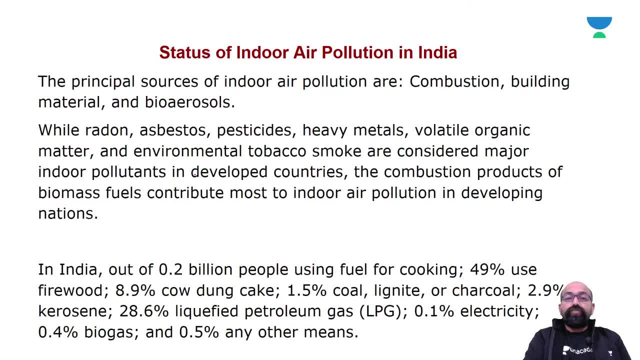 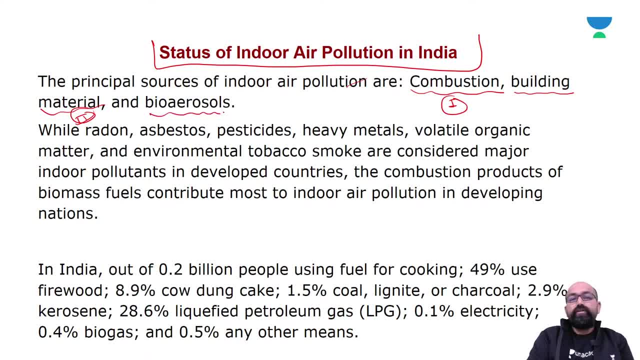 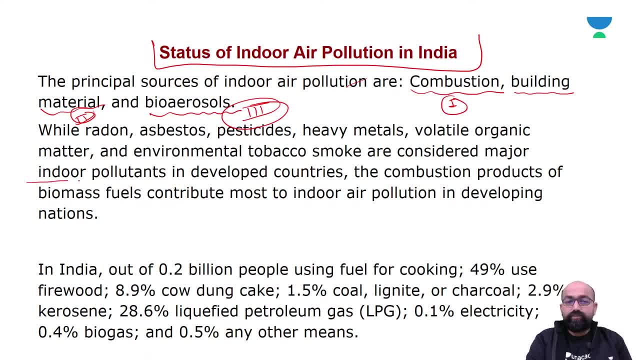 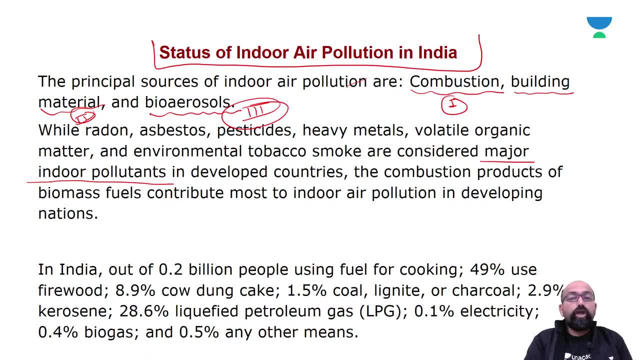 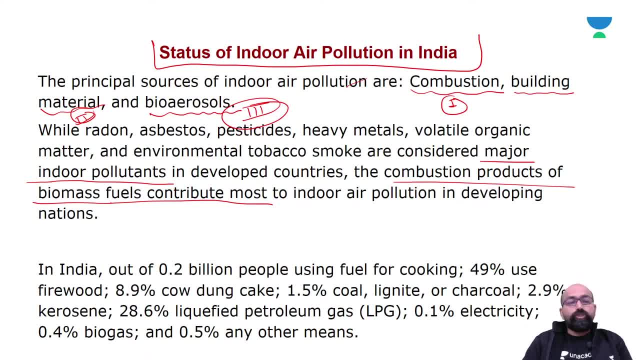 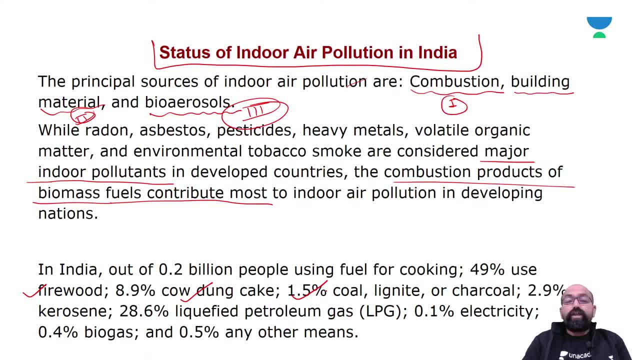 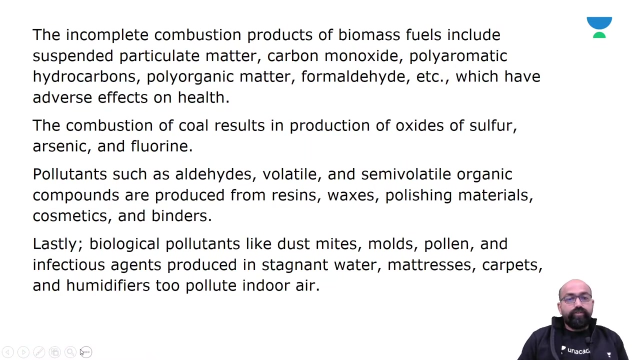 Okay, Okay, Okay, Okay. gas, that is LPG, point one percent electricity, point four percent biogas and point five zero, point five percent other methods: yes, so we will see all these different flat platforms or methods used for cooking in India which are also responsible for the indoor air pollution. yes, so the incomplete 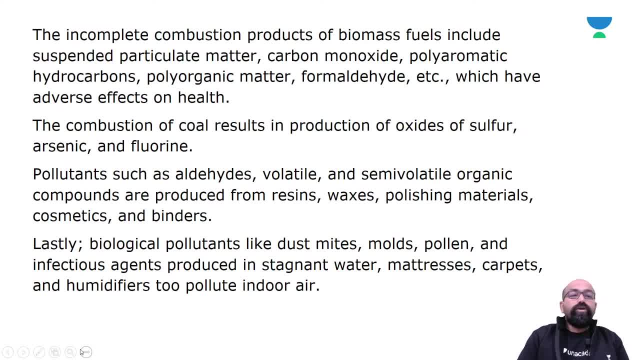 combustion of products of biomass. fuels include suspended particulate matter, carbon, carbon monoxide, poly aromatic hydrocarbons, poly organic matter for formaldehyde, etc. which have adverse effects on health. yes, the combustion of coal results in production of oxides of sulfur, arsenic and fluorine. yes, the combustion of coal results in production of oxides of. 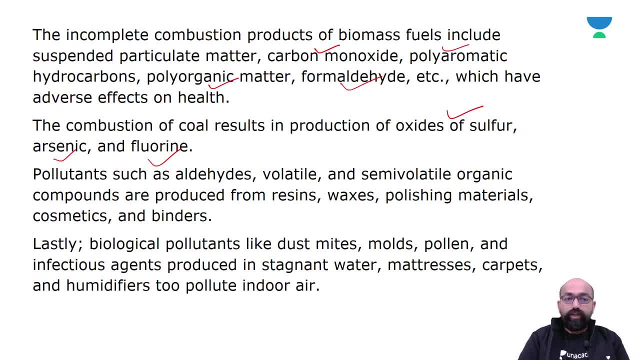 sulfur, arsenic and fluorine. now pollutants such as aldehydes volatile. semi-volatile organic compounds are produced from resins, waxes, polishing materials, cosmetics and binders. yes, the combustion of coal results in the production of oxides of sulfur, arsenic and fluorine. now pollutants such as aldehydes volatile. 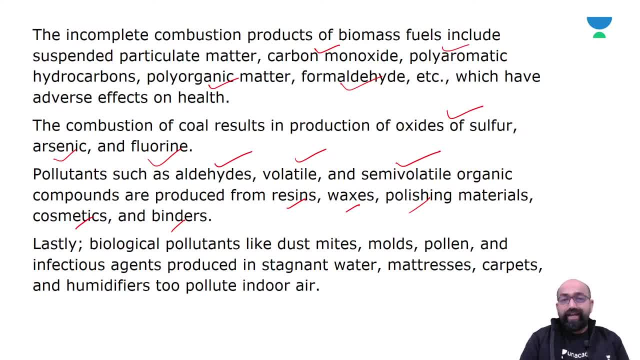 semi-volatile organic compounds are produced from resins, waxes, polishing materials, cosmetics and binders. yes, the combustion of coal results in the production of oxides and living minerals, such as deploying hydrogen, akt and so on. so not everything is production based on organic nitrogen. let us see how our finished. 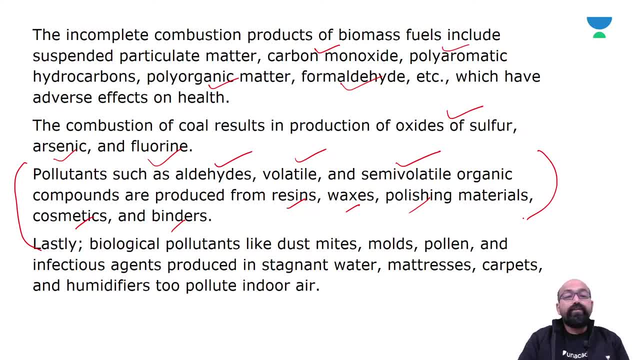 த流 sliced pet bulkhead compared to little simple próxima past. now see our state to day activities. how affected the air quality? yes, so the pollutants, such as aldehyde, volatile and semi-volatile organic compounds are produced from resins, waxes, polishing materials, cosmetics and binders. and finally, biological pollutants, like carcinogens, if you like to talk about how to solve the pollution of carcinogens andına. 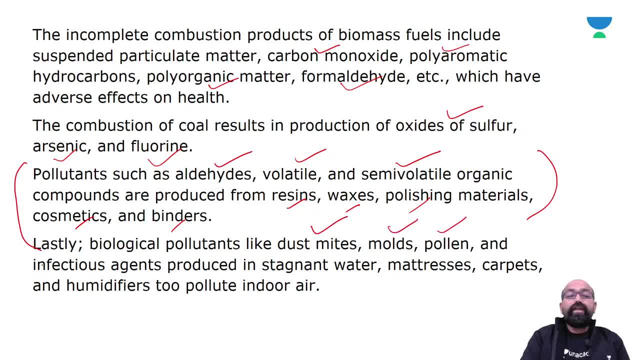 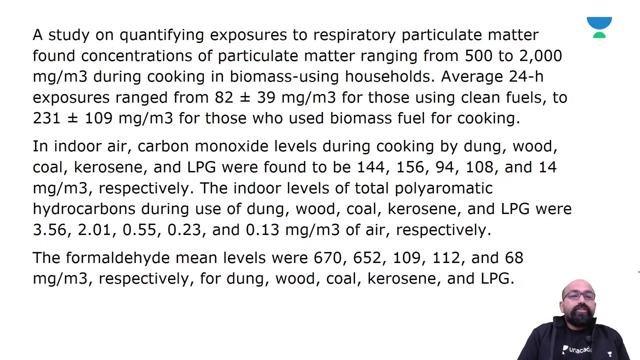 dust mix, moulds, pollen and infectious agents produced in stagnant water, mattress, carpets and humidifiers to pollute indoor air. So all these factors are responsible for indoor air pollution? Yes. after that, a study on quantifying exposures to respiratory particulate matter found concentration. 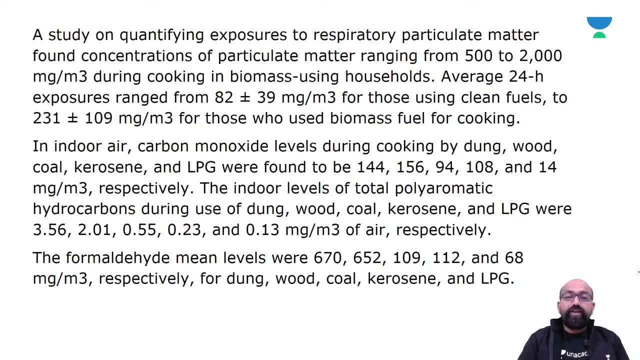 of particulate matter ranging from 500 to 2000 mg per m3 during cooking in biomass or using households, So average 24 hours a day. Mass exposures ranged from 82 ± 39 mg per m3 for those using clean fuels to 231 ± 109. 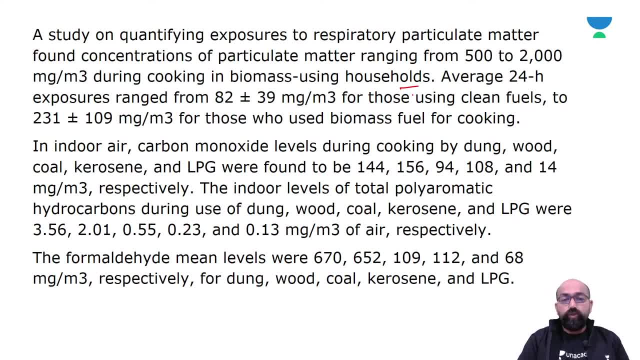 mg per m3 for those who used biomass fuel for cooking. Yes, so indoor air carbon monoxide levels during cooking By dunk wood, coal, kerosene and LPG were found to be 144,, 156,, 94,, 108 and 14 mg m3 respectively. 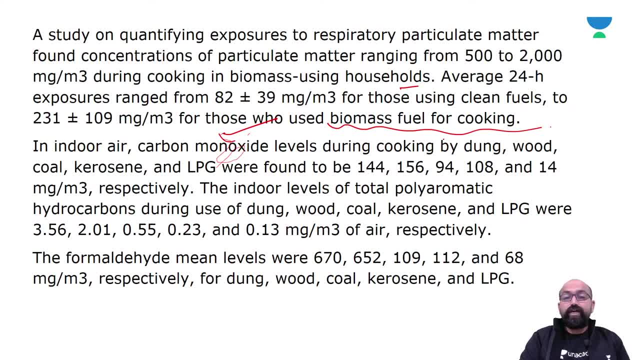 Yes, So cooking by dunk 144, wood 156, coal 94, kerosene 104 and LPG were found to be 144,, 156,, 94,, 108 and 14 mg m3 respectively. Yes, So cooking by dunk 144, wood 156, coal 94, kerosene 104 and 14 mg m3 respectively. 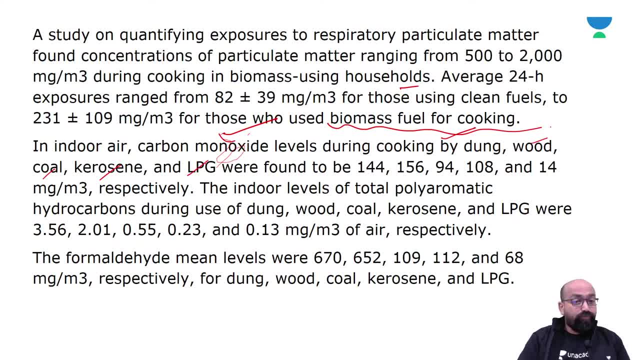 Yes, So the outdoor levels of total polyaromatic hydrocarbons during use of dunk wood, coal, kerosene and LPG were 3.56,, 2.01,, 0.55,, 0.23, and 0.13 mg per m3 of air respectively. 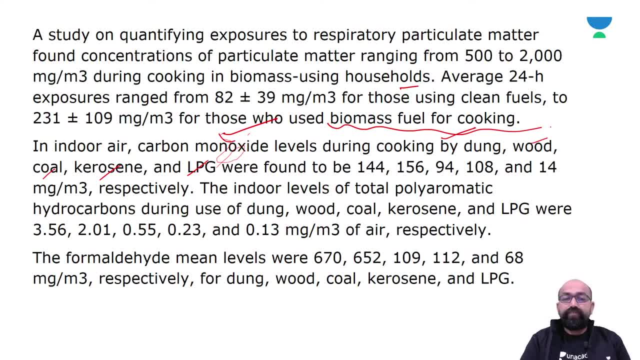 Yes, So these are the indoor levels of total polyaromatic hydrocarbons during the use of dunk wood coal. kerosene and LPG were 3.56,, 2.01,, 0.55,, 0.23, and 0.13 mg per m3 of air respectively. 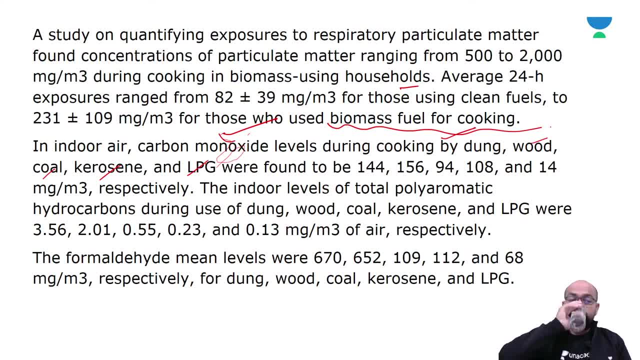 Yes, the formaldehyde means levels were 670, 652, 109, 112 and 68 mg per m3 respectively for dunk wood, coal, kerosene and lpg. see, these are the measurement methods and the figures which calculated to through air. indoor air pollution: yes, after that we'll see effects of indoor air. 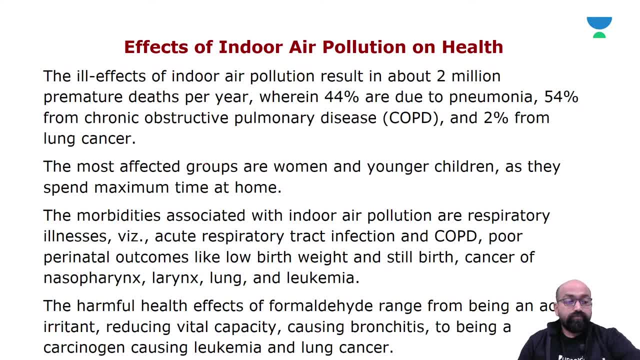 pollution on health. yes, so the ill effects of indoor air pollution results in about 2 million pre-mature deaths per year, wherein 44 percent are due to pneumonia, 54 percent from chronic obstructive pulmonary disease- copd- chronic obstructive pulmonary disease- and 2 from lung cancer. yes, this is the data approximate related with the effects. 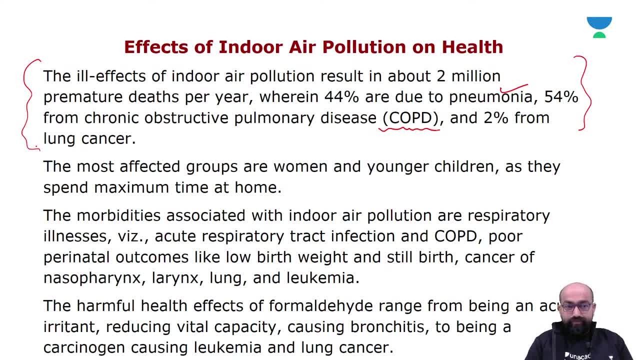 of indoor air pollution on health. now the most affected groups are women and younger children, as they spend maximum time at home. so the mobilities effects on legs and ribs is that in the morning 8 see these. all these Mobilities associated with indoor air pollution are respiratory illness, acute respiratory tract infection and COPD, chronic obstructive pulmonary disease. poor perinatal outcomes like low birth weight, stillbirth, cancer of nasopharynx, larynx, lung and leukemia. 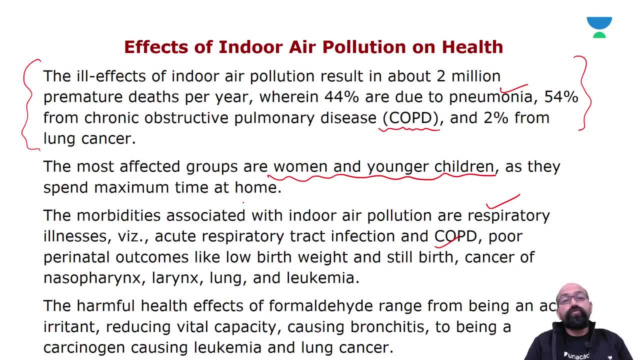 Yes, friends, these are the effects of indoor air pollution on health. Along with that, the harmful health effects of formaldehyde range from being an acute irritant reducing vital capacity, causing bronchitis, to being a carcinogen, causing leukemia and lung cancer. 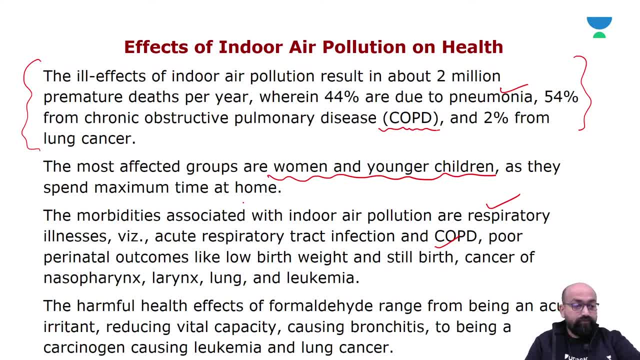 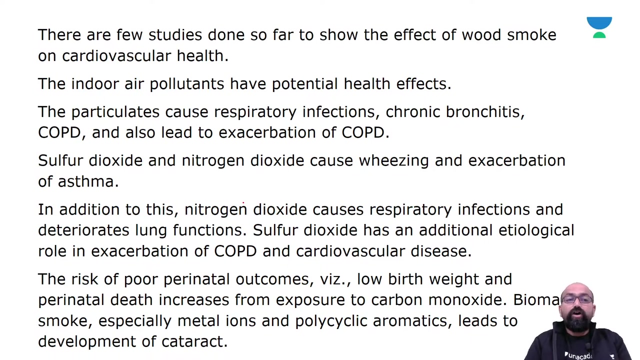 Yes, Yes, guys. So So the harmful health effects of formaldehyde range from being an acute irritant reducing vital capacity, causing bronchitis, to being a carcinogen causing leukemia and lung cancer. Now there are a few studies done so far to show the effect of wood smoke on cardiovascular health. 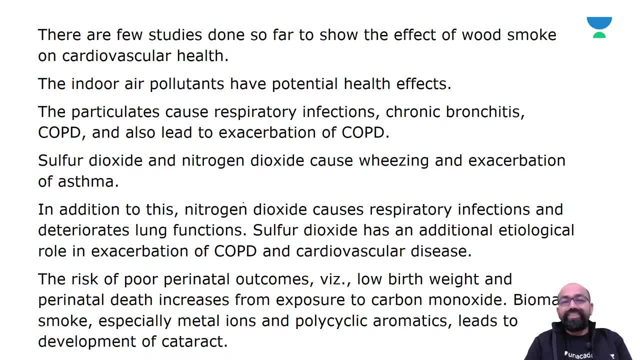 Yes, the indoor air pollutants have potential health. Like the particulates, cause respiratory infections, chronic bronchitis, COPD, and also lead to X- X accretion of COPD. Yes, So basically sulfur dioxide: Yes, 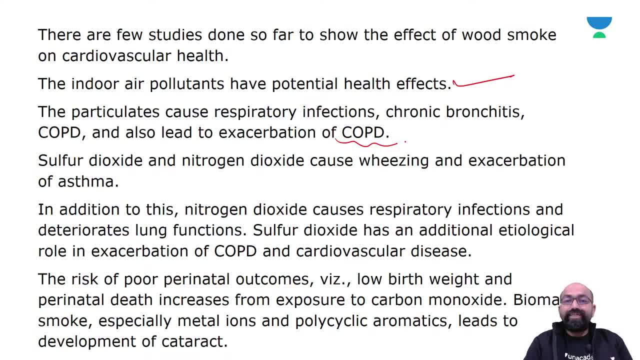 Sulfur dioxide. and nitrogen dioxide causes wheezing and X accretion of asthma. So, in addition to this, nitrogen dioxide causes respiratory infections and deteriorates lung functions, Sulfur dioxide has additional. It's your logical role in X, the revision of COPD and cardiovascular disease. 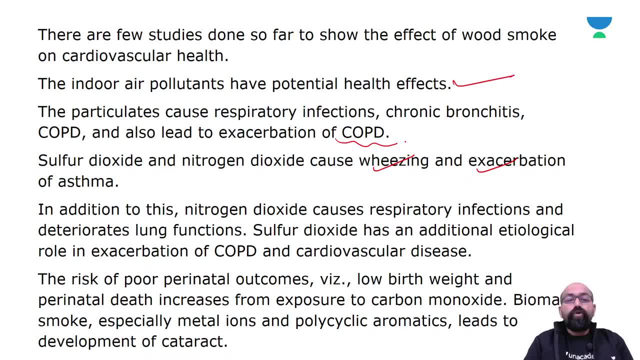 Yes, So the risk of poor perinatal outcomes, that is, low birth weight and perinatal death, increases from exposure to carbon monoxide, biomass, smoke, smoke, especially metal ions, and polycyclic aromatics, Leads to development of cataract. 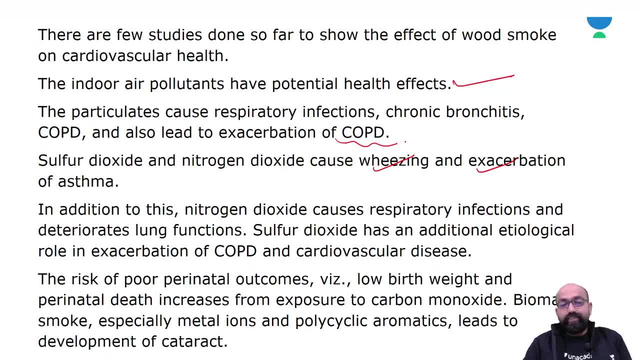 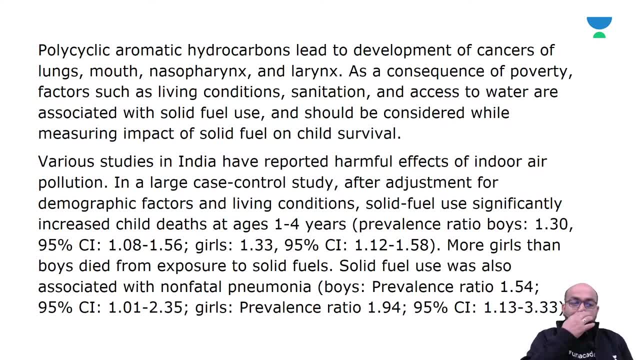 Yes, guys. So these are the effects of air pollution on indoor air pollution on health. Now, polycyclic aromatic hydrocarbons lead to development of cancers of lungs, mouth, nasopharynx and larynx. So, as consequent, 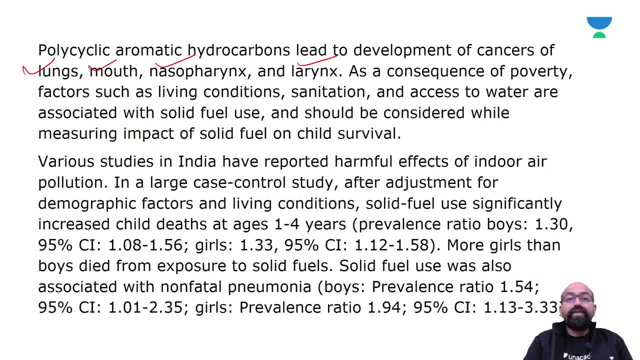 of poverty. factors such as living conditions, sanitization and access to water are associated with the solid fuel use and should be considered while measuring impact of solid fuel on child survival. So various studies in our country have reported harmful effects of indoor pollution. So in a large case control study after adjustment for democratic factor and living conditions. 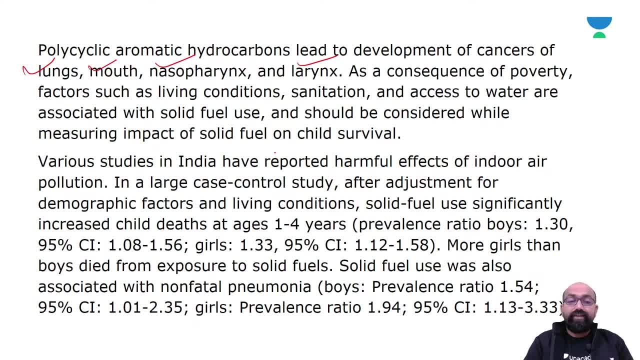 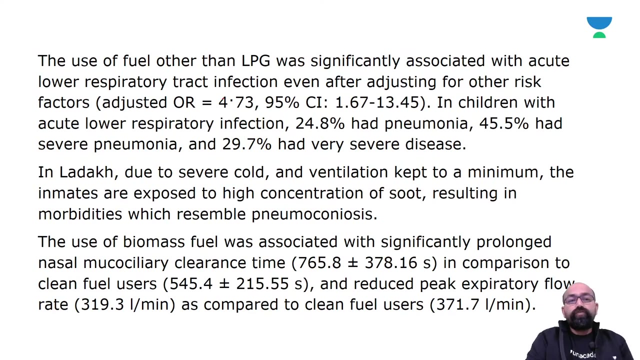 solid fuel use significantly increased child deaths at ages 1 to 4 years. Yes, more girls than boys died from exposure to solid fuels, and solid fuel use was also associated with non-fatal pneumonia. Yes, guys, So the use of fuel other than LPG was significantly associated with acute lower respiratory tract. infection, even after adjusting for the for other risk factors. So in children, Yes, With acute lower respiratory infection, like 24.8% had pneumonia, 45.5% had 7 pneumonia and 29.7% had very severe disease. 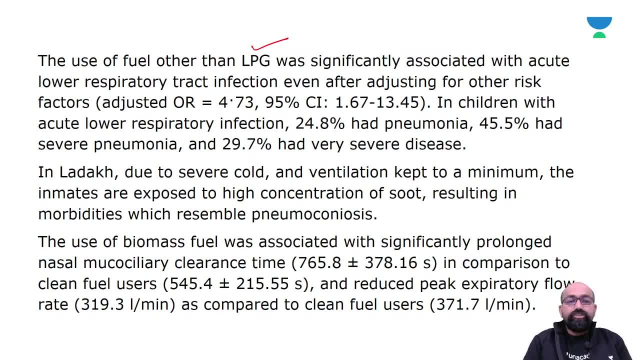 Yes, So if we'll see. in Ladakh, due to severe cold and ventilation kept to a minimum, the inmates are exposed to high concentration of soot, So the use of fuel was associated with significantly prolonged nasal mucociliary clearance time in comparison to clean fuel. 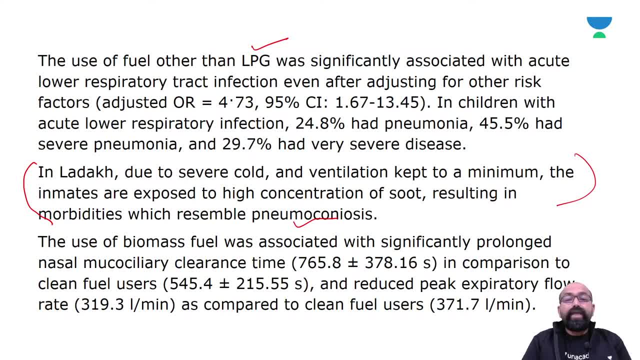 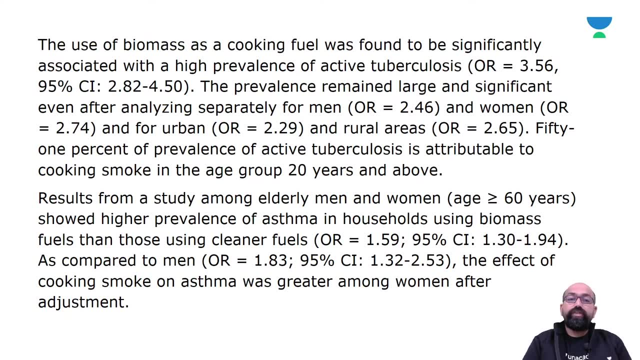 Clean fuel uses and reduced peak expiry rate flow rate as compared to clean fuel uses. So the use of biomass as a cooking fuel was found to be significantly associated with high prevalence of active tuberculosis. yes, tuberculosis right. the prevalence of prevalence remained large. Yes, This is significant, even after analyzing separately for men and women and for urban and rural. 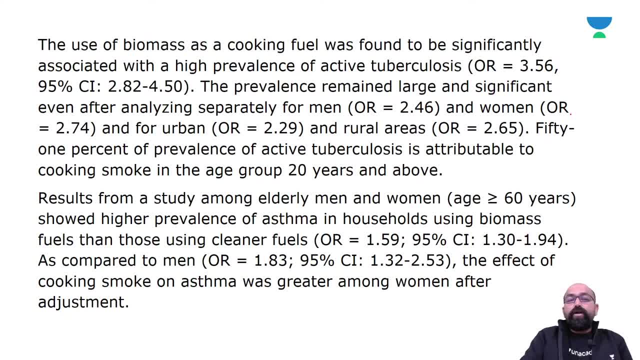 areas. So 51% of prevalence of active tuberculosis is attributable to cooking smoke. in the age of group 20 years and above. Yes, So results from a study among elderly men and women showed higher prevalence of active tuberculosis. Yes, Yes, Due to the worst incidence of asthma in household using biomass fuels than those using cleaner. 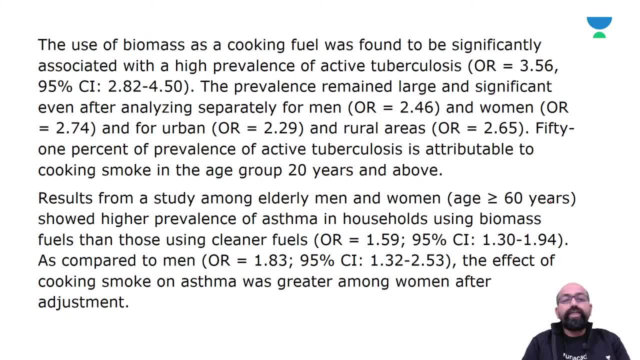 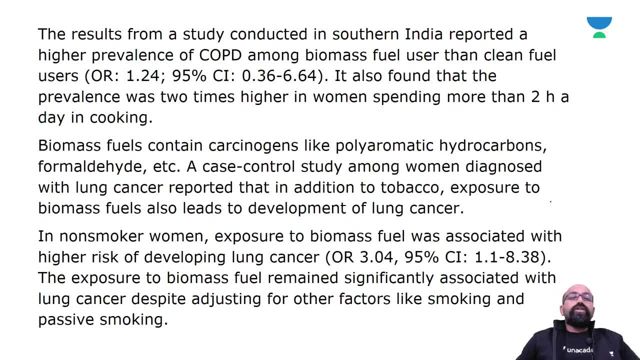 fuels as compared to men, and the effect of cooking smoke on asthma was greater among women after adjustment. Yes, So the reason from a study conducted in southern India reported higher prevalence of COPD among biomass fuel user than clean fuel users. Yes, Yes. 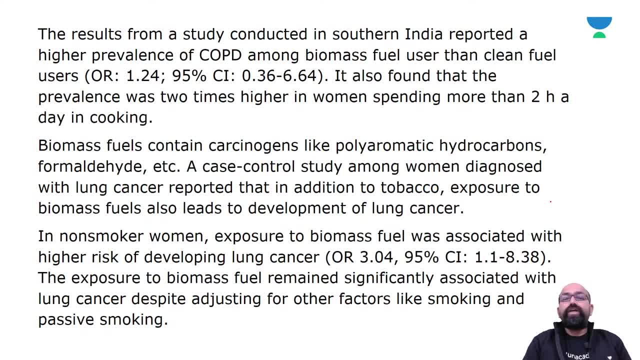 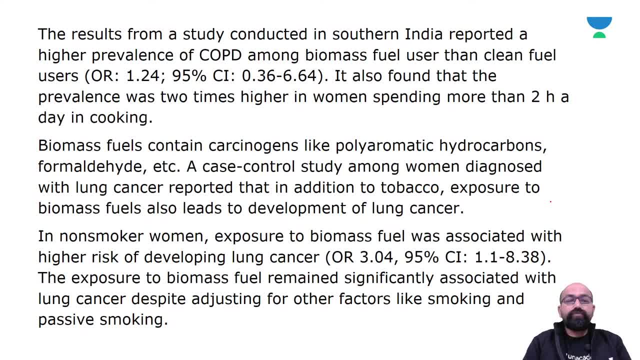 in addition to tobacco, exposure to biomass fuels also also leads to development of lung cancer. right so, in non-smoker women, exposures to biomass fuel was associated with higher risk of developing lung cancer, and the exposure to biomass fuel remained significantly associated with lung cancer despite adjusting for other factors like 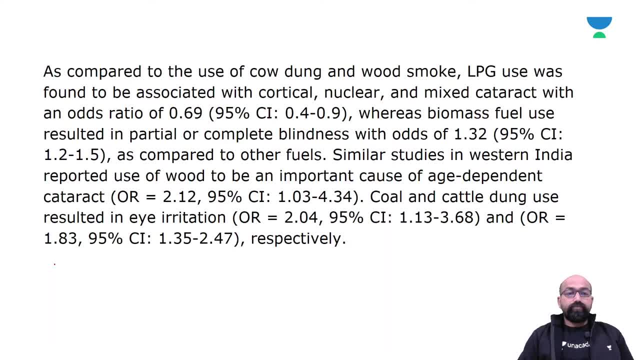 so smoking and passive smoking, yes, so these are the factors related with the indoor air pollution on health. now along continuing with this event. compared to the use of cow junk and wood smoke, lpg use was found to be associated with cortical, nuclear and mixed cataracts with an odd ratio of 0.69, whereas biomass fuel use resulted in partial or complete. 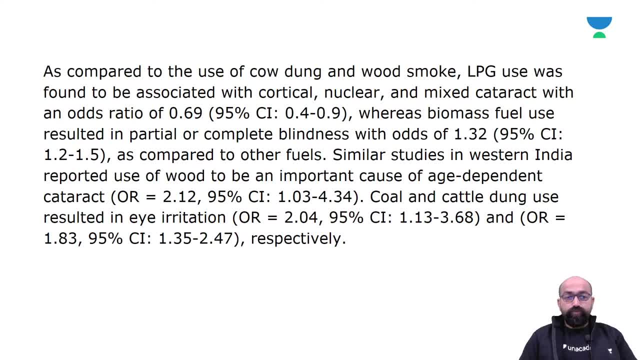 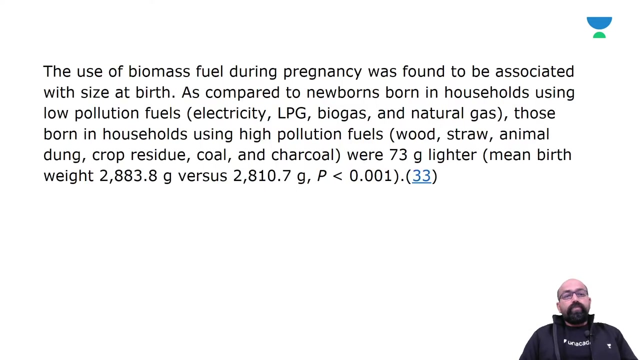 blindness with odds of 1.32 as compared to other fuel. so similar studies in western india reported use of wood to be an important cause of age-dependent cataract. yes, coal and cattle done use resulted Eyes irritation a yes, Supalım Produced vegetables High. 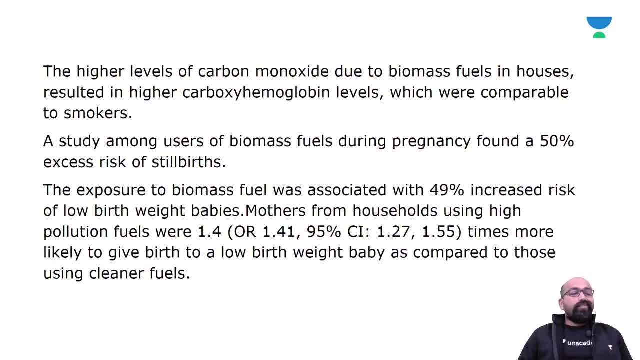 certified nutrients. one fermentation of admires solid want possible. Hey, Please share these appropriate materials for drinking you. Suitable, clean, squ. MEL veut higher carboxyhemoglobin levels which were comparable to smokers. yes, and a study among users of biomass fuels during pregnancy found a 50 percent excess risk of. 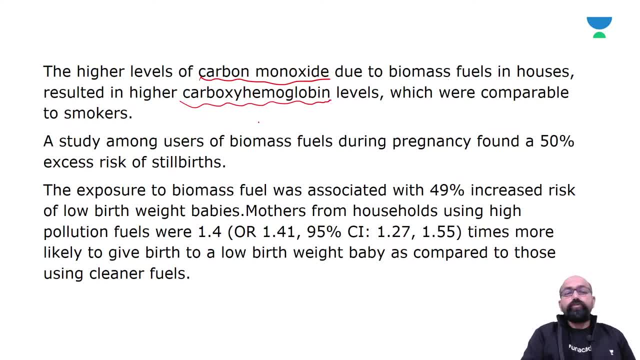 stillbirths right. so the exposure to biomass fuel was associated with 49 percent increased risk of low birth wet babies. so mothers from household using high pollution fuels were 1.4 times more likely to give birth to a low birth weight baby as compared to those using cleaner fuels. yes, so the 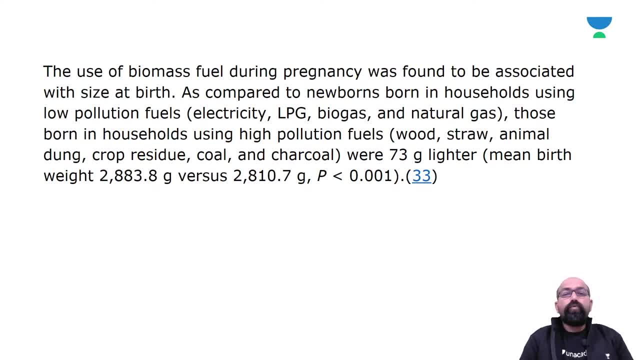 use of biomass fuel during pregnancy was found to be associated with at birth and, as compared to newborn or newborns born in households using low pollution fuels like electricity, lpg, biogas and natural gas, those born in households using high- full high pollution fuels where 73g lighter 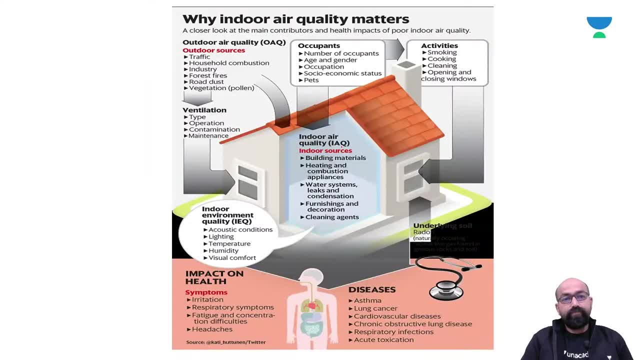 right, yes, now see this picture is talked about indoor air quality matters. yes, now what we have theoretically studied about health impact on health or health impact of poor indoor air quality- just have a look in this picture. so, yes, so indoor air quality. so indoor sources, building materials, heating and combustion appliances. 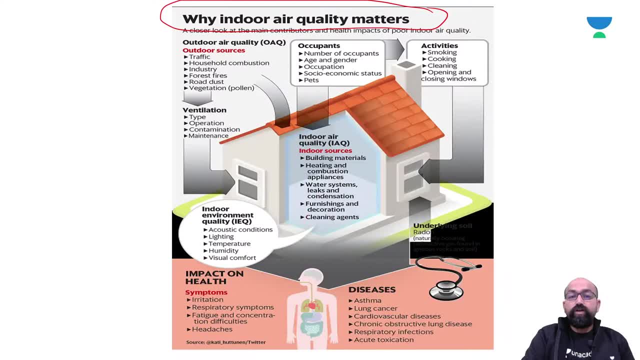 water systems, leaks and condensation, furnishing and decoration. cleaning agents: yes. now, indoor environment quality- ieq is acoustic condition, lightning, temperature, humidity and visual comfort- yes, okay, occupants like number of occupants, age and general occupation. social economic status and pates: social economic status in house. in house. 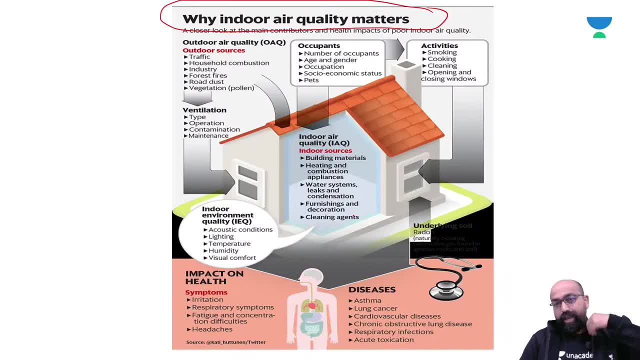 s in house: Yes, and if we are talking about activities like smoking, cooking, cleaning, opening and closing windows: Yes. endo impact on health, like symptoms: irritation, respiratory symptoms, fatigue and concentration difficulties, headaches: Yes. diseases: asthma, lung cancer, cardiovascular disease, chronic obstructive lung disease, respiratory infections and acute toxication. 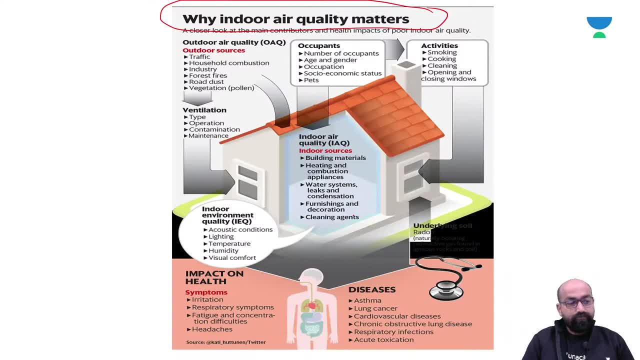 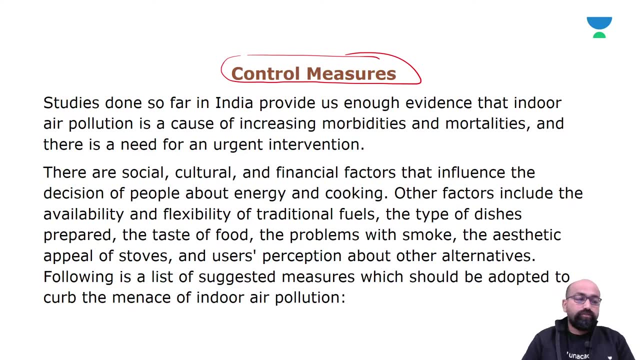 Yes, Now, after that, we'll see control measures for endoimpact Indoor air pollution. Yes, friends, So this- The studies done so far in our country- provides us enough evidence that indoor air pollution is a cause of increasing morbidity, morbidity and mortality. 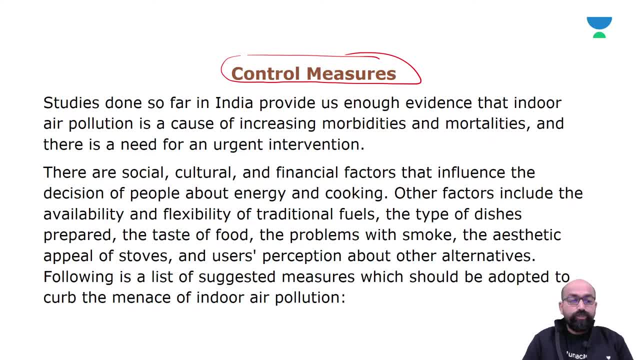 And there is a need for an urgent intervention. So there is Social, Cultural and financial factors that influence the decision of people about energy and cooking. So other factors include the availability and flexibility of traditional fuels, the type of dishes prepared, the test of food, the problems with smoke, the aesthetic apples of stores and users perception about other alternatives. 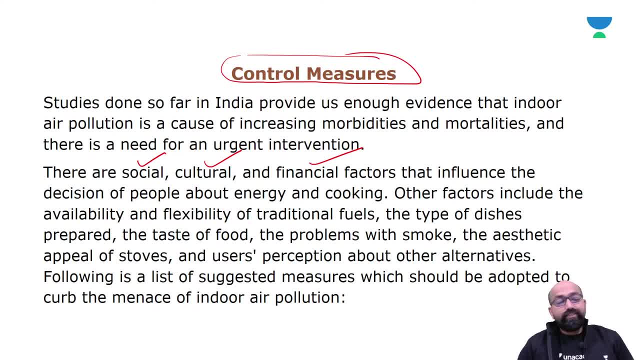 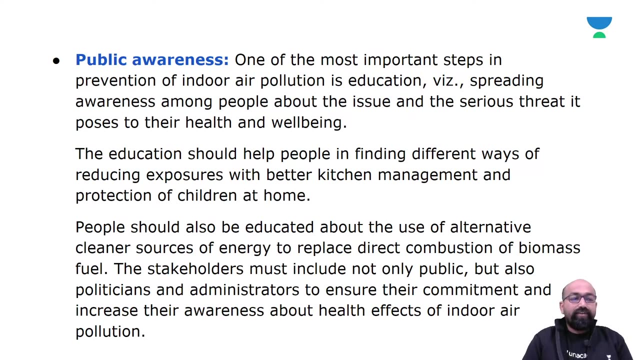 Yes, So we'll see the suggested measures which should be adopted to curb the menace of indoor air pollution. Yes, So where? First is public awareness Right? So one of the most important steps In prevention of indoor air pollution is education. 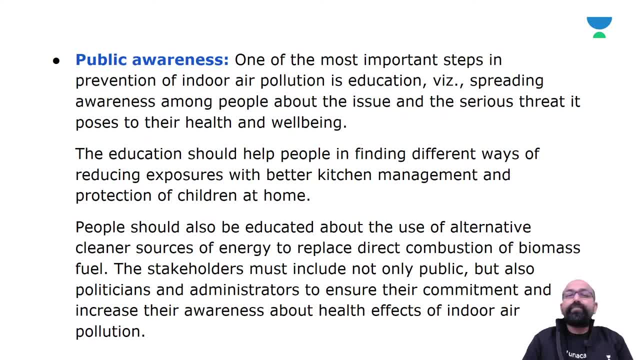 Yes, Spreading awareness among people about the issue and the serious state It poses that health and well-being. So public awareness is important. Measure- Yes, Then, which includes the education should help people in finding different ways of reducing exposures, with better kitchen management and protection of children at home. 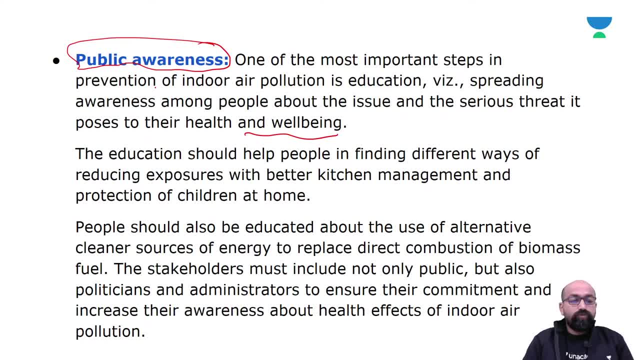 So people should also Be educated about the use of alternative, cleaner sources of energy to replace direct combustion of biomass fuel. The stakeholders must include not only public but also politicians and administrators, to ensure their commitment and increase their awareness about health effects Of indoor air pollution. 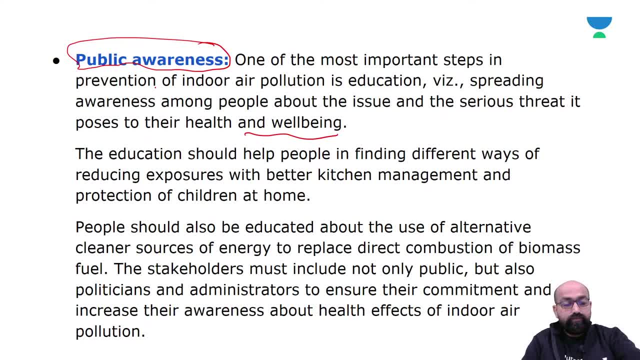 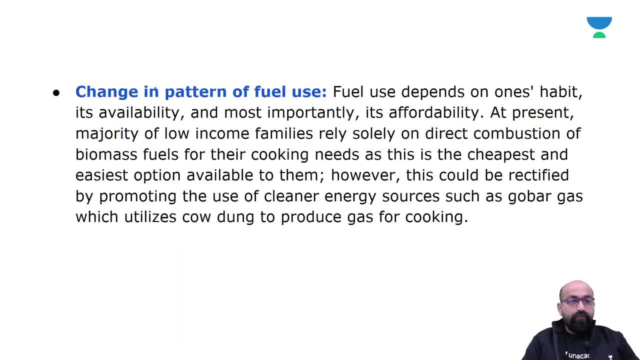 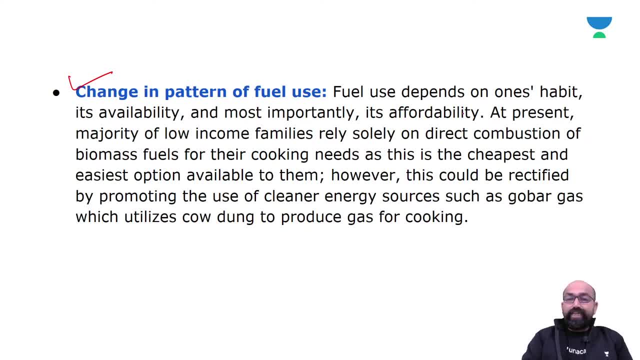 So fuel use depends on one's habit and availability And, most importantly, its affordability. So at present, Majority of low income families- families- rely solely on direct combustion of biomass fuels for their cooking needs, as this is the cheapest and easiest option available to them. 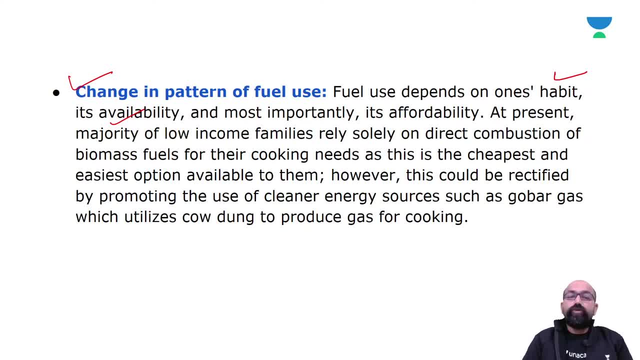 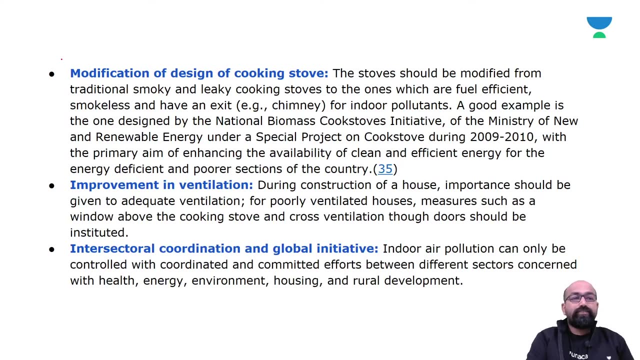 However, this could be rectified by promoting the use of cleaner energy sources, such as goba gas, which utilizes cow dung to produce gas for cooking. Next, modification of design of cooking stoves: The stoves should be modified from traditional smoky and leaky cooking stoves to the ones 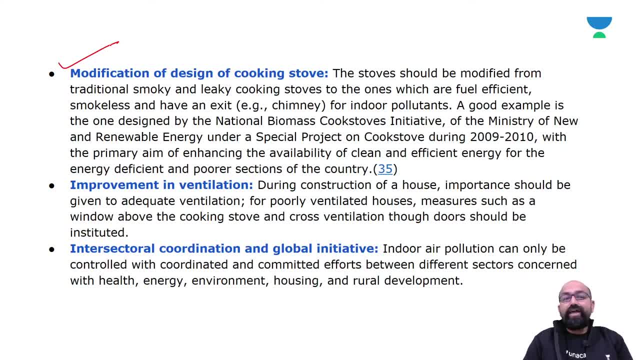 which are fuel efficient, smokeless and have an exit that is chimney for indoor pollutants. A good example is one designed by National Biotech Corporation. Next, modification of design of cooking stoves: The initiatives of the Ministry of New Renewable Energy under a special project on cook stoves. 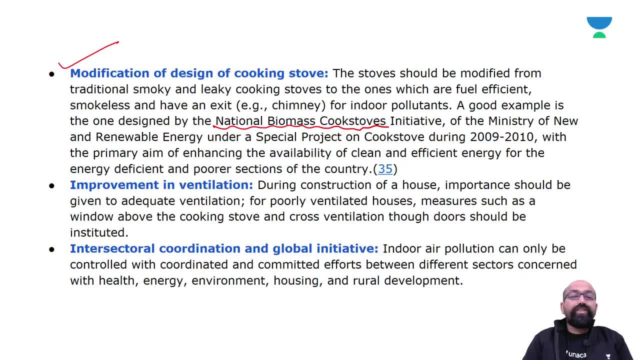 during 2009 and 2010.. So, with the primary aim of enhancing the availability of clean and efficient energy for the energy-deficient and poorer sections of the country, Yes, modification of design of cooking stoves, Then improvement in ventilation. 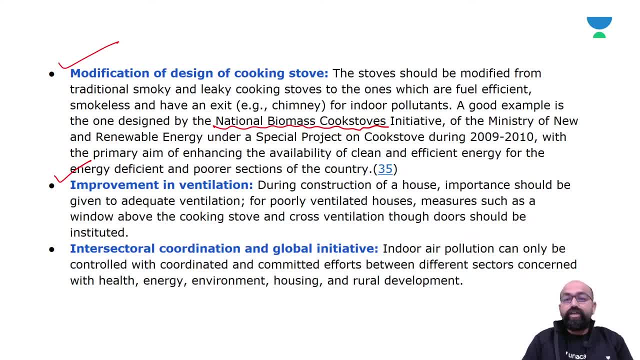 So, during construction of a house, importance should be given to adequate ventilation for poorly ventilated houses, measures such as a window above the cooking stove and cross ventilation through doors which be instituted. Yes, ventilation is also important to reducing indoor air pollutant during cooking. 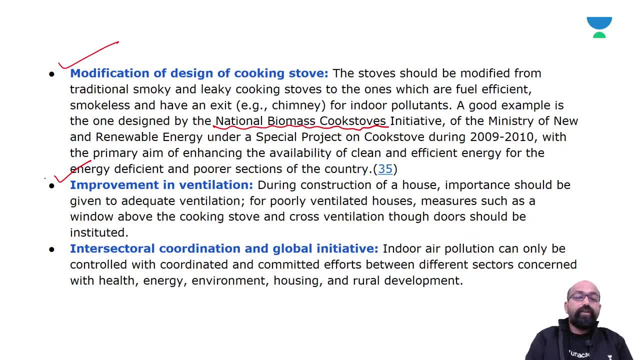 Then inter-sectoral coordination and global initiative. Yes, so indoor air pollution can only be controlled with coordinated and committed efforts between different sectors concerned with health safety and safety With energy, environment, housing and rural development. Yes, now, after that we will see. 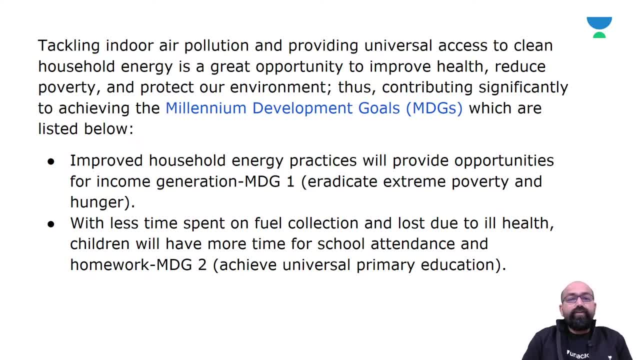 Millennium Development Goals. Yes, Yes, Yes, Right. So tackling indoor air pollution and providing universal access to clean household energy is a great opportunity to improve health, reduce poverty and protect our environment, Thus contributing significantly to achieving the Millennium Development Goals. 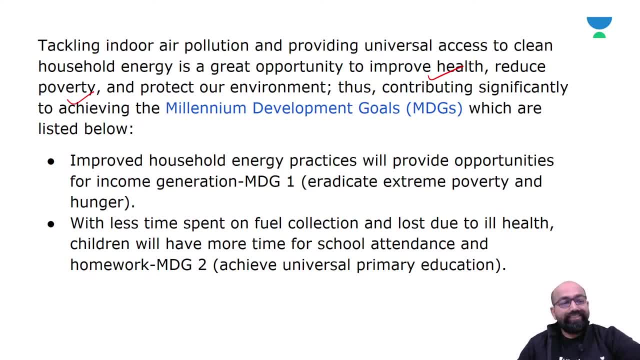 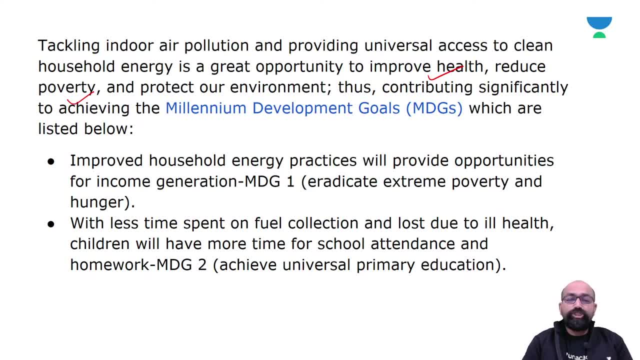 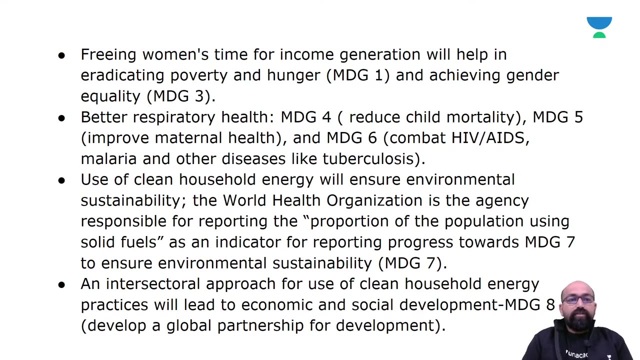 and homework, which is the mdg. to achieve universal primary education: yes, first is eradicate extreme poverty and hunger. second one: achieve universal primary education. then freeing women's time for income generation will help in eradicating poverty and hunger and achieving gender equal education equality. yes, guys. 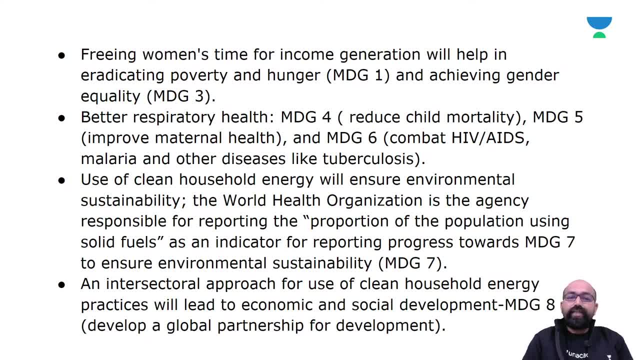 better respiratory health. yes, mdg4, which reduce child mortality. mdg5 improve maternal health. sixth, combat HIV and AIDS, malaria and other diseases like tuberculosis. then use of clean household energy will ensure environmental sustainability. so the WHO is the agency responsible for reporting the proportion of population using solid fuels. 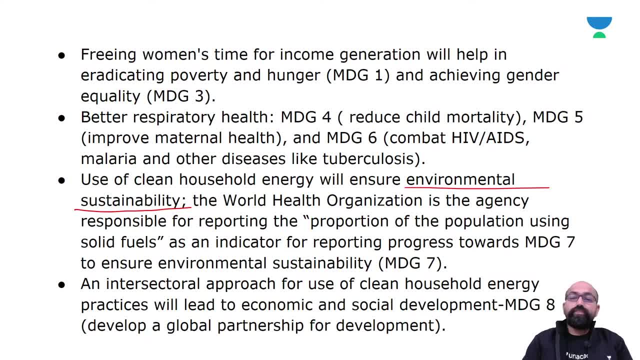 as an indicator for reporting progress towards mdg7 to ensure environmental sustainability. MDG 7 and an inter-sectoral approach for use of clean household energy practices will lead to economic and social development. so develop a global partnership for development. yes, so though, if it is. 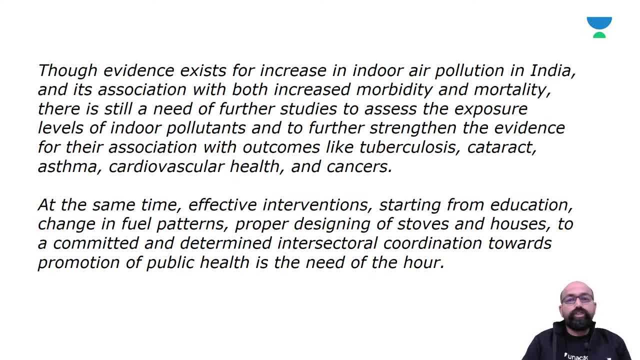 exists for increasing air pollution in India and its association with both increased mobility and mortality. so there is still a need of further studies to assess the exposure levels of indoor pollutants and to further send in the evidence for their association with outcomes like tuberculosis, cataract, asthma. 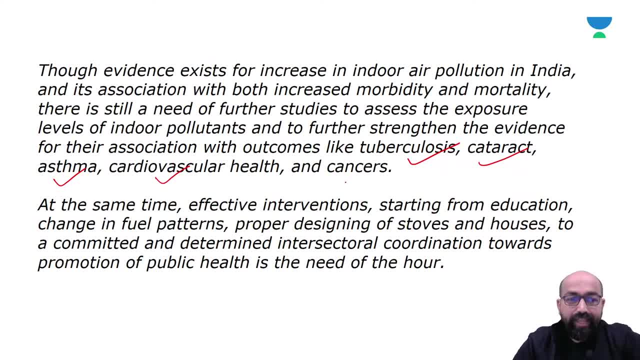 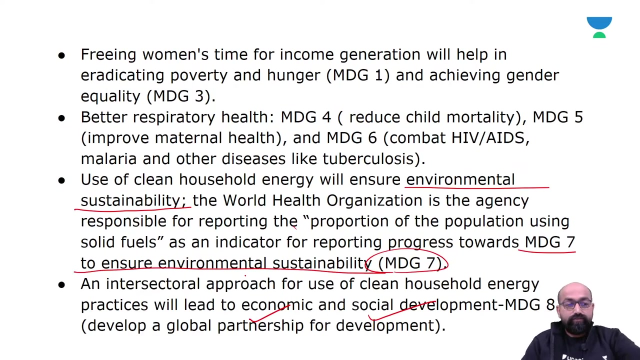 and cardiovascular health and cancers. so, at the same time, effective interventions starting from education, change in fuel pattern, change in fuel patterns, proper designing of stores and houses, to a committed and determined inter-sectoral coordination towards promotion of public health, is the need of the arm. yes, 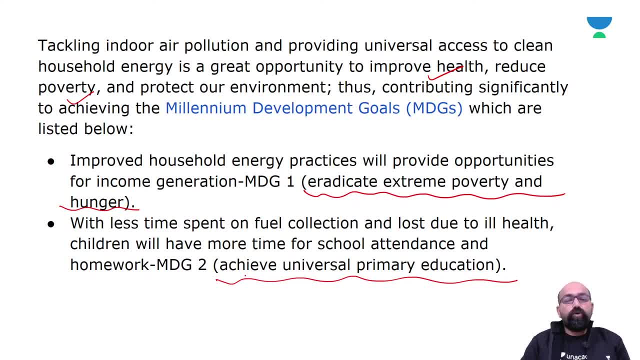 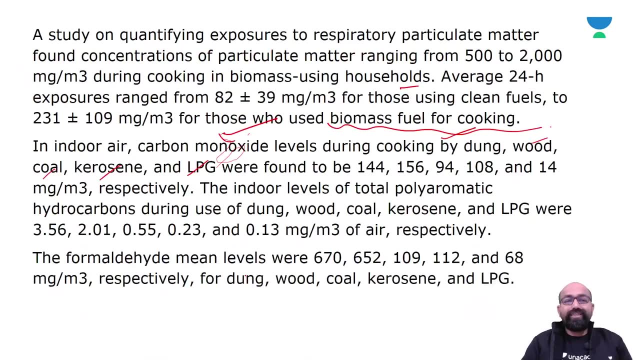 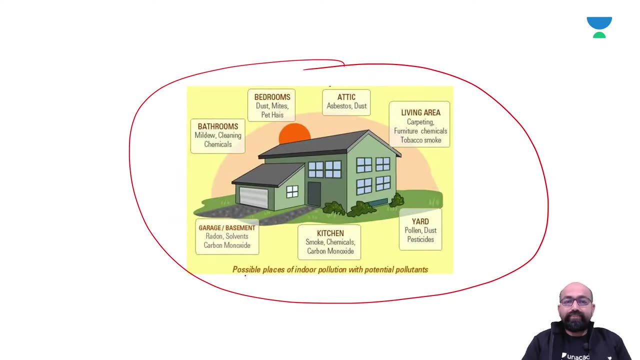 so these are the millennium development goals and conclusion of how to control indoor air pollution. so, friends, just have a recap what we have covered in today's lecture. indoor air pollution, yes, yes. now see the factors related to this. the first: corssic, atic asbestosis and dust. if we are talking about lieutenantır giden ins, undercover04 governments of the country. 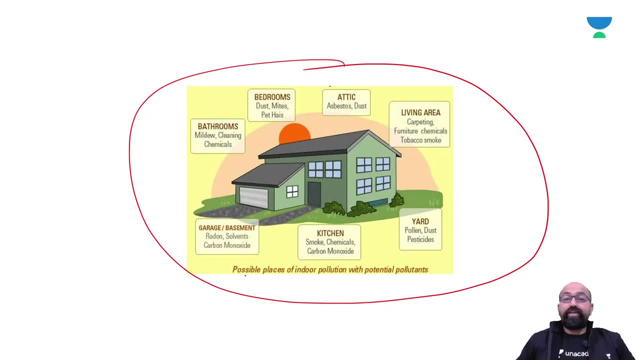 dust. if we are talking about the living area, than carpenting furniture chemicals, tobacco smoke. bedrooms like dust mites, potholes, bathrooms, mildew cleaning chemicals. garage or basement like radios, solvents, carbon monoxide, kitchen smoke chemicals, carbon monoxide. yes, these are the possible places. 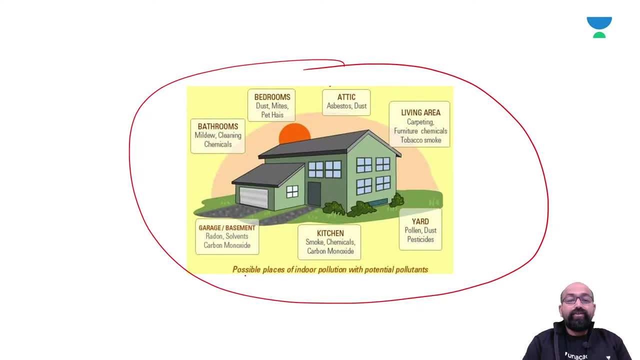 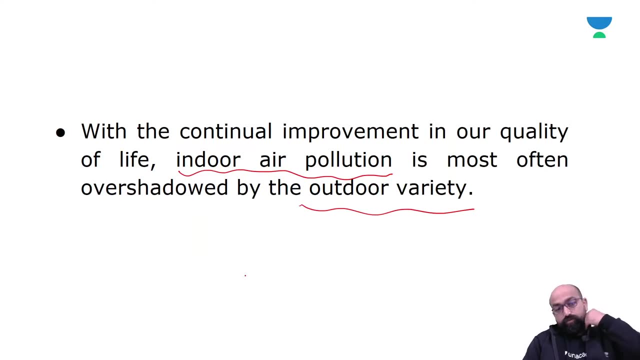 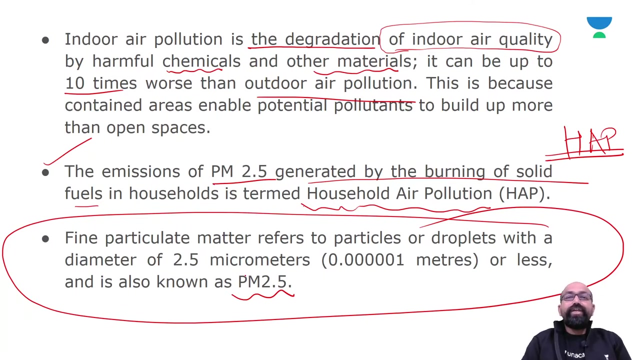 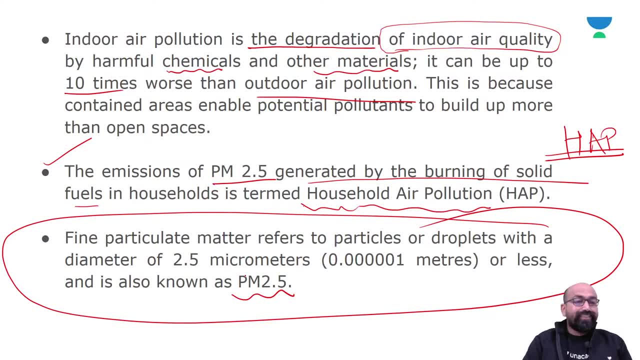 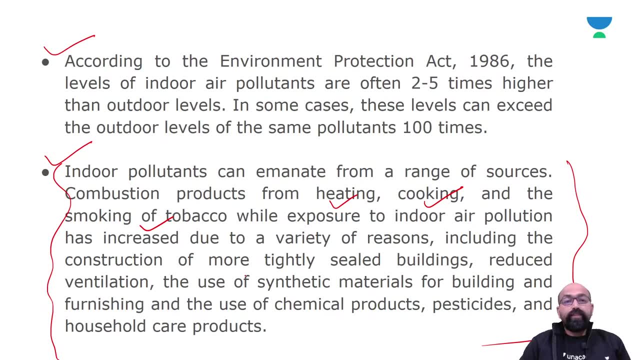 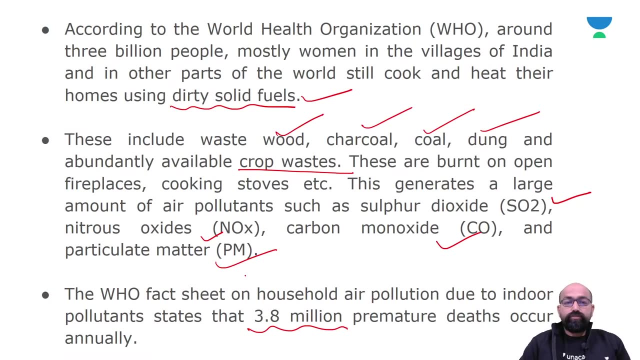 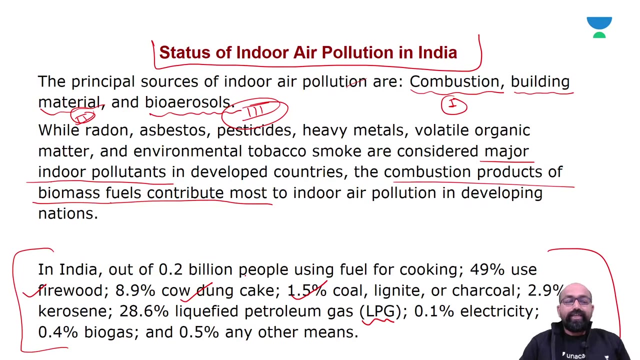 carbon monoxide are generated by the burning of solid fuels in household. in terms of household air pollution HAP. Yes, then we have covered all the information related with the indoor air pollution and the related various factors to that. Yes, then we have covered status of indoor air pollution in India. 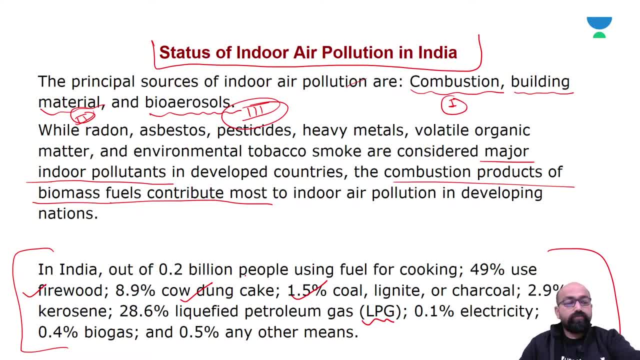 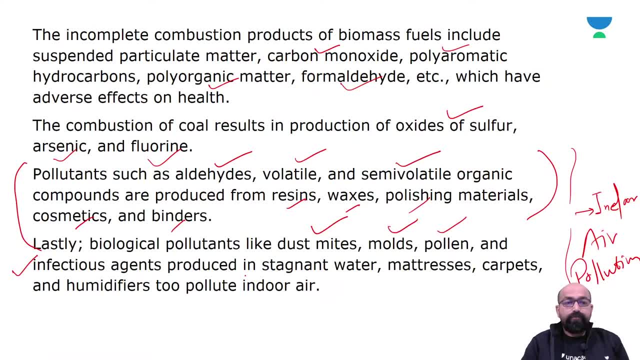 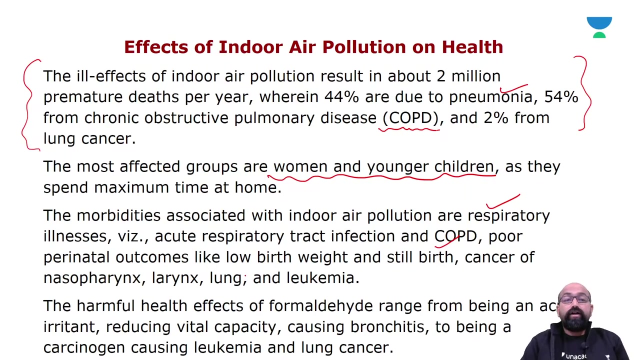 Yes, so basically the pollutants like aldehydes, volatile and semi-volatile organic compounds are produced from resins, waxes, polishing materials, cosmetics and binders, And also indoor air pollutants, Then we have studied few facts and figures related to harmful effects of indoor air pollution. 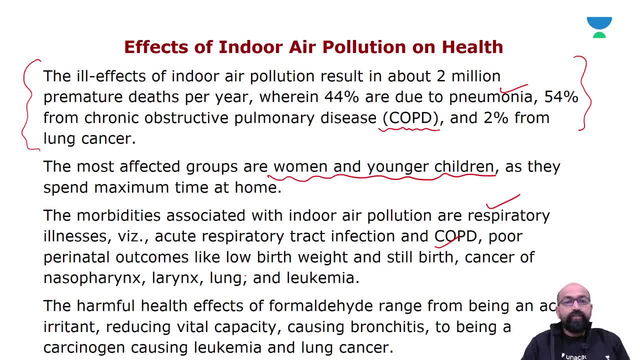 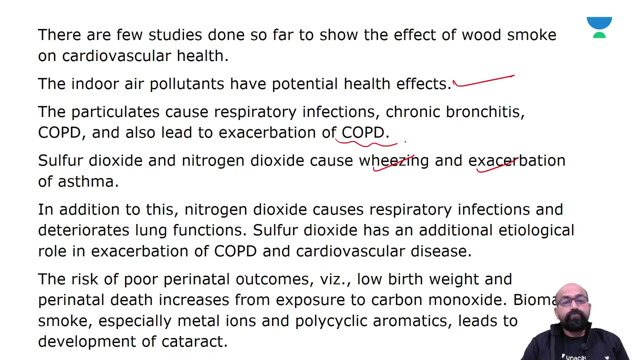 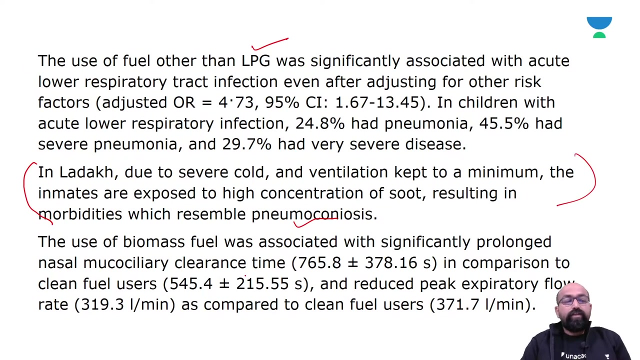 on Health. Yes, so these are the effects on health, like Pneumonia, Tronic obstructive pulmonaryк disease, COPD, lung cancer and many more. yes, Then we have studied the example of Ladakh, where, due to severe cold and ventilation kept to a minimum, the inmates 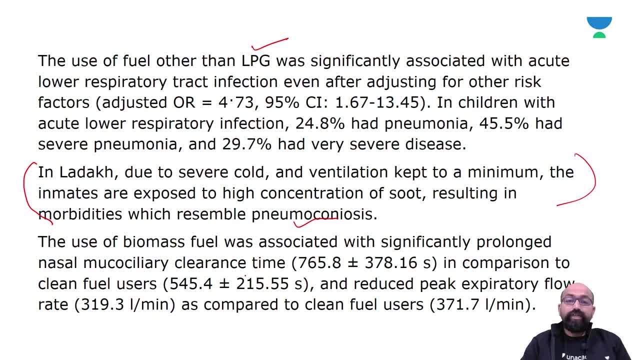 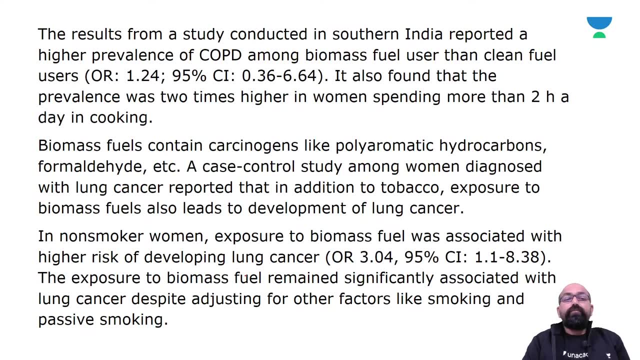 are exposed to high concentration of soot, resulting in morbidities which resemble pneumoconiosis. Yes, and biomass fuels contain carcinogens like polyaromatic hydrocarbons, formaldehyde, and a case control study among women diagnosed with lung cancer reported that, in addition to tobacco, exposure to 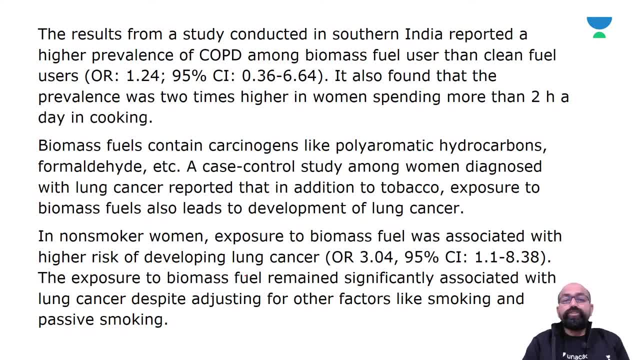 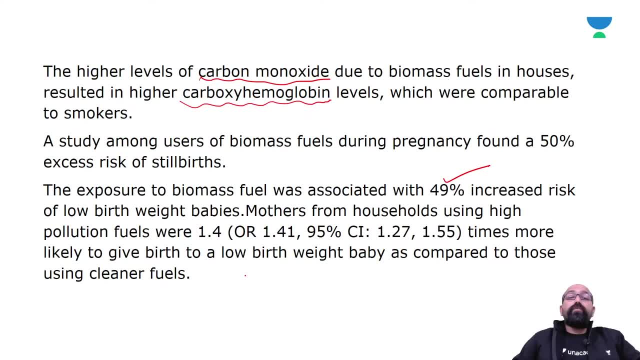 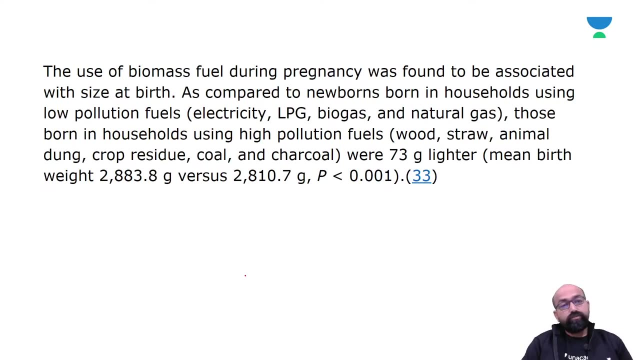 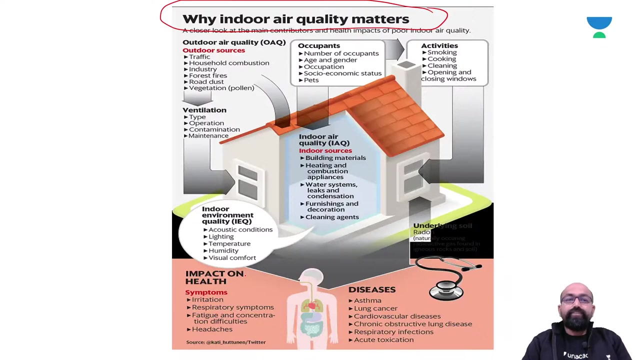 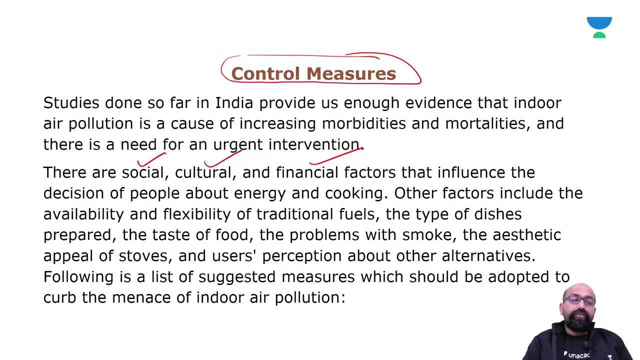 biomass fuels also leads to development of lung cancer. Yes, the higher levels of carbon monoxide due to biomass fuels in houses resulted in higher carboxyhemoglobin levels, which were comparable to smokers. and then we have seen the picture. why indoor air quality matters? Yes, and then we have covered. 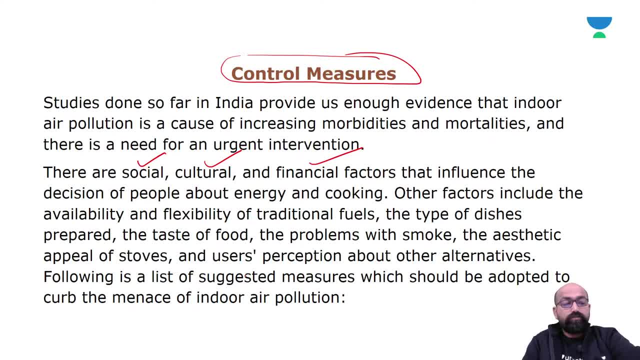 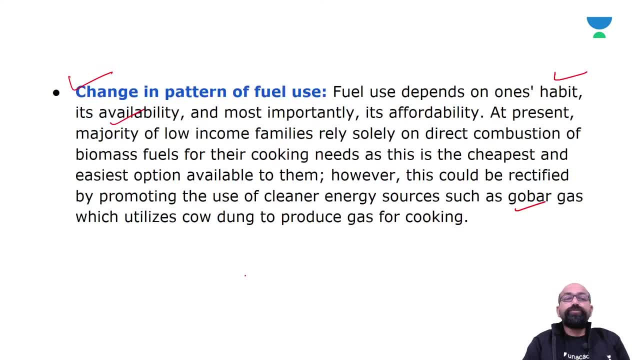 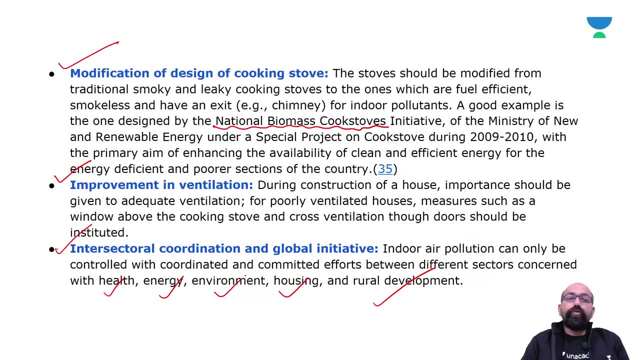 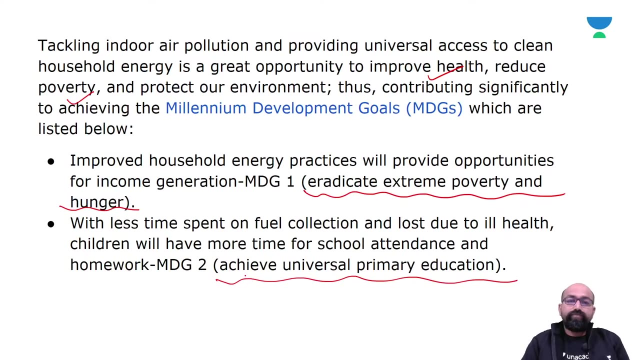 control measures: Yes. public awareness, change in pattern of fuel, fuel use, modification of design of cooking stove, improvement in ventilation, Inter-sectoral coordination and global initiative: Yes. Then we have said how to contributing to achieving the achieving the Millennium Development Goals. 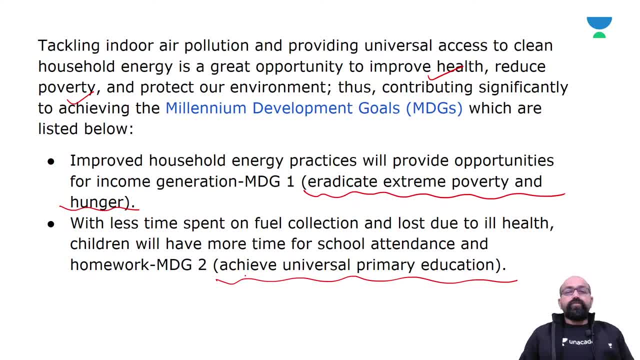 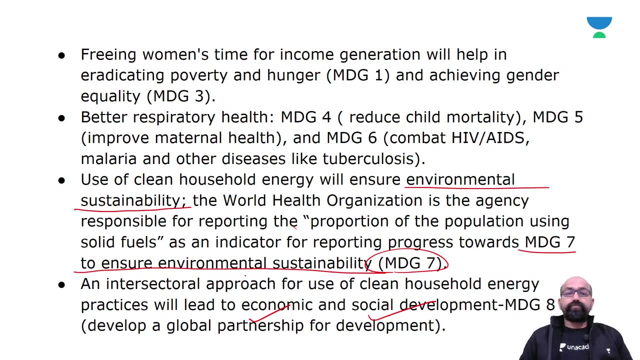 MDGs: Yes, where, first, eradicate extreme poverty and hunger. second, achieve universal primary education. Achieving gender equality. Fourth, reduce child mortality. Fifth, improve maternal health. Sixth, combat HIV, AIDS, malaria and other diseases like tuberculosis. Yes, Then, to improve gender equality First leads to understand the environmental